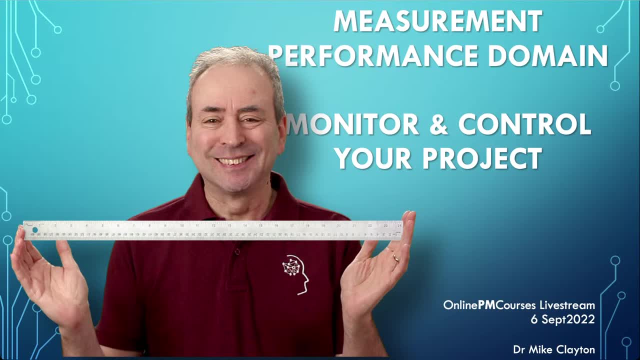 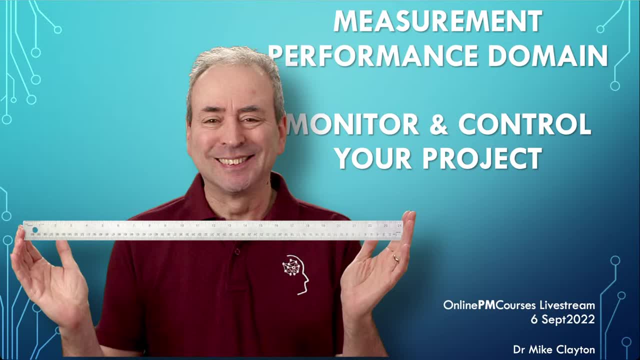 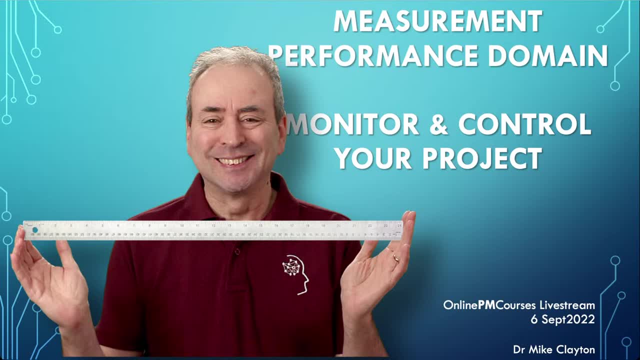 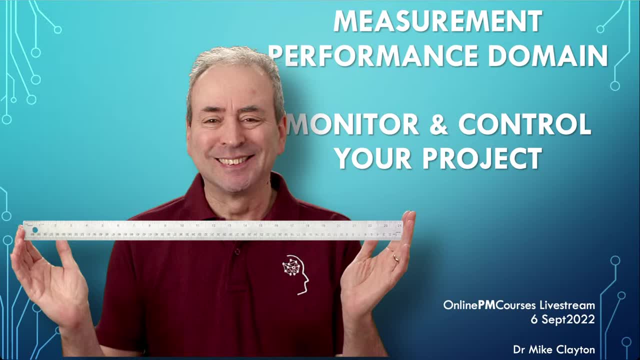 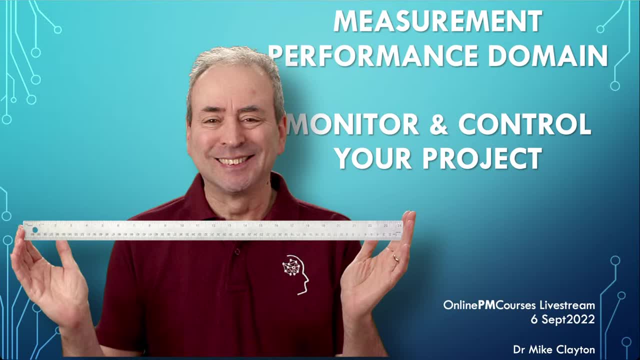 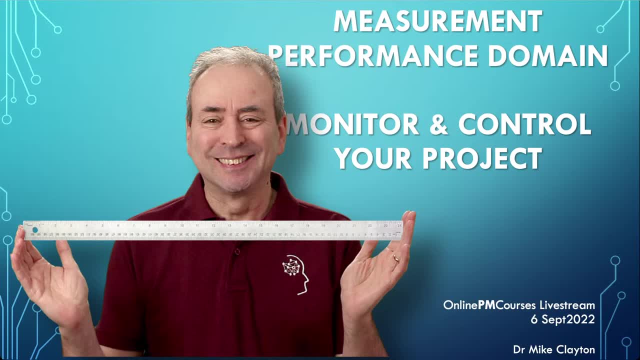 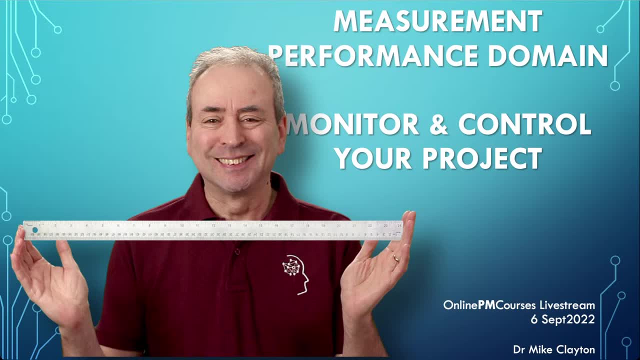 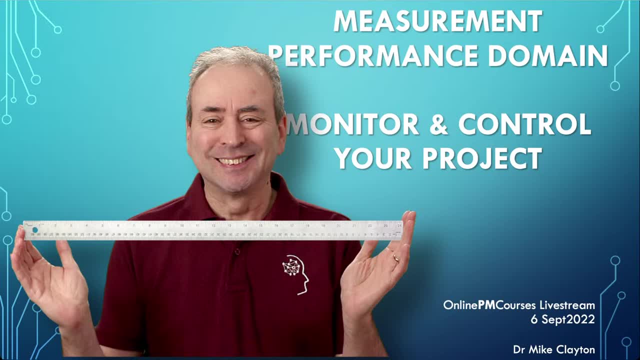 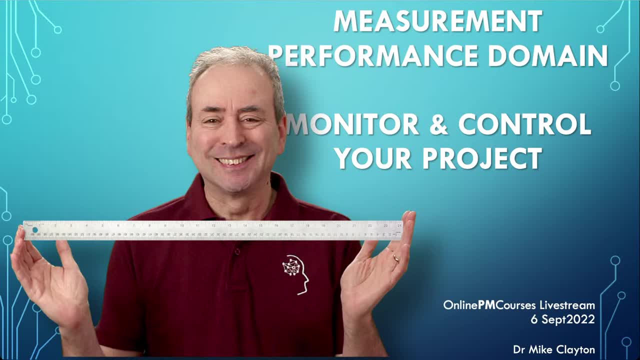 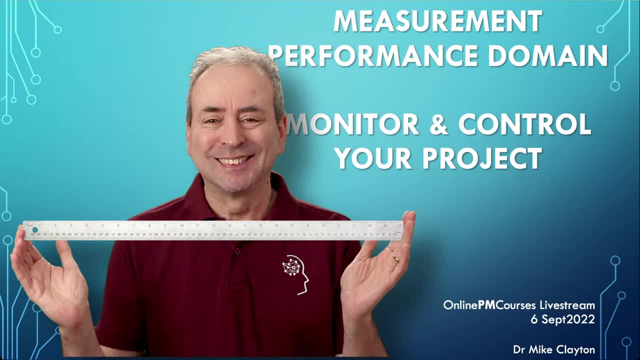 boulder, okori emmanuel. um good, i'm still getting stream status poor and loads of errors uh, flooding my youtube studio um the analytics. yeah, i, yeah. it looks like four or four people have dropped off the stream in the last five minutes, so i'm a bit worried, but we will carry on. 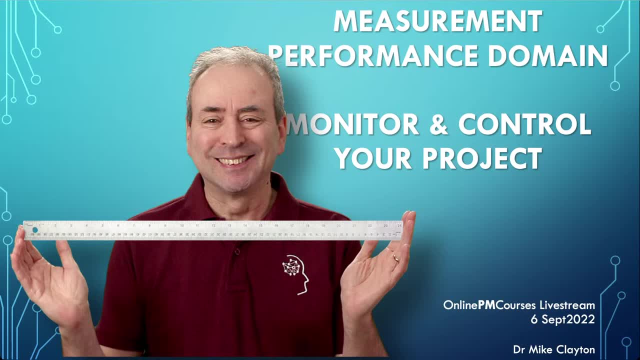 until i get confirmation through the chat that, uh, you're having a bad time and it's not worthwhile, i will carry on. um, so what we're going to do today is look at the seventh of the eight performance domains from the penbot guide. as usual, we're just going to. 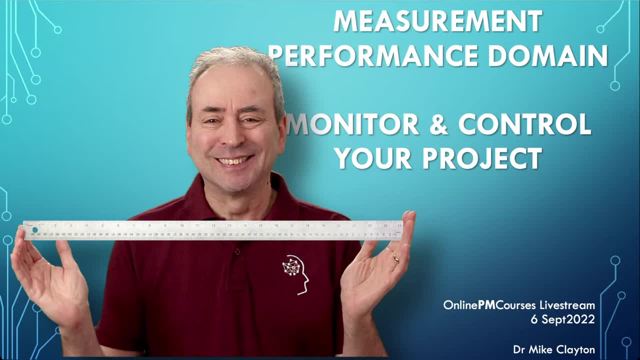 i'm going to go through them one by one. so we're going to go through them one by one. and then we're going to go through them one by one. so we're going to go through them one by one. just going to use that as a an opportunity and a kicking off point, not, uh, i'm not going to go. 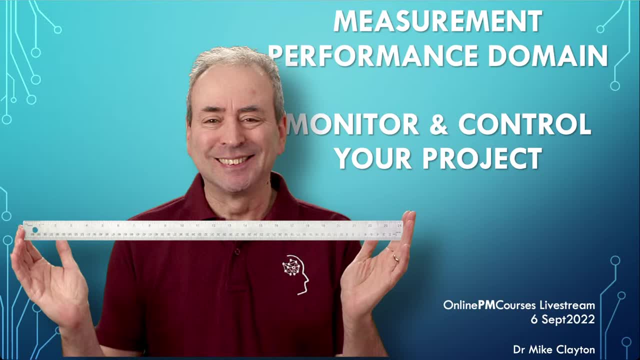 through the pinball guide. i'm wondering, maybe one day, uh, whether to do that, but certainly not today. we're going to look at monitoring control, which, for me, is the heart of the delivery stage of a project. it's where we're doing all our monitoring, all our measurements, so that's what we're going to focus on. 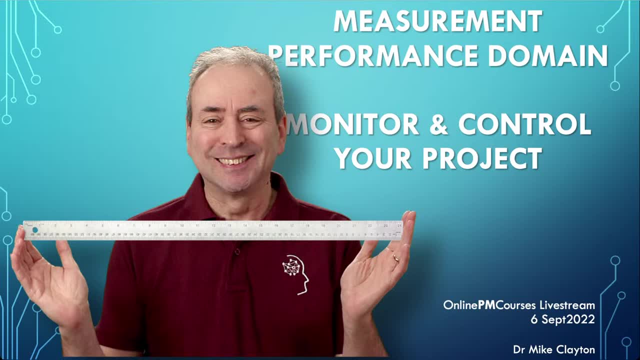 uh, what else? um, i'm also at the end of this session can tell you what the next two are, because the next one, uh, obviously will be the last of our performance domain- uh, deep dives. but i've actually lined up the november uh stream, which is going to be something a bit special. i. 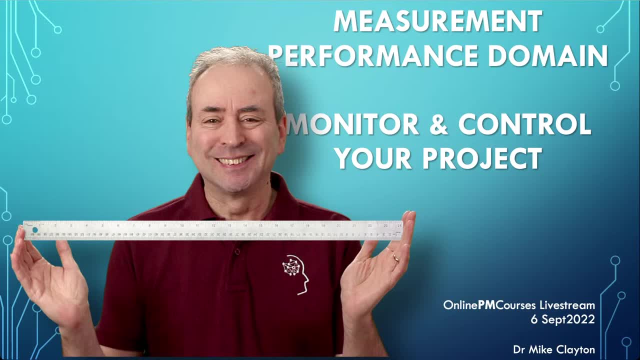 hope. um, uh, edwin, good audio from my end, from bonnie island, nigeria. wow, that's, that's three people from nigeria. that's brilliant. uh, obviously time zones isn't a problem for you guys, because you're, i think, an hour or so ahead of us. um, uh, then, uh, patrick uh from the us. hello, patrick uh todd from orlando, florida. audio video is: 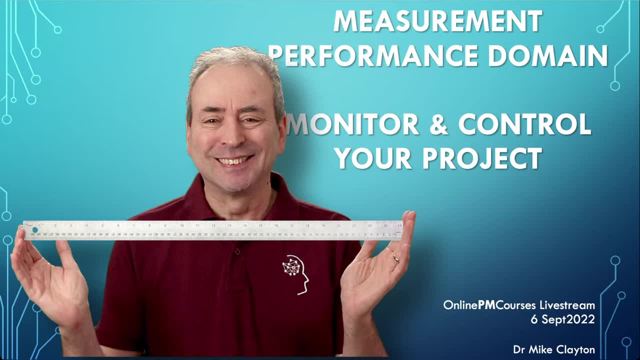 adequate, i'll take adequate. and then we've got tunde ade uh, who is a kind of regular contributor to the channel. um, great to see, uh, great to see you there. um, i'm kind of uh, um glad to see so many familiar faces and so many new faces. it's great to have that balance. 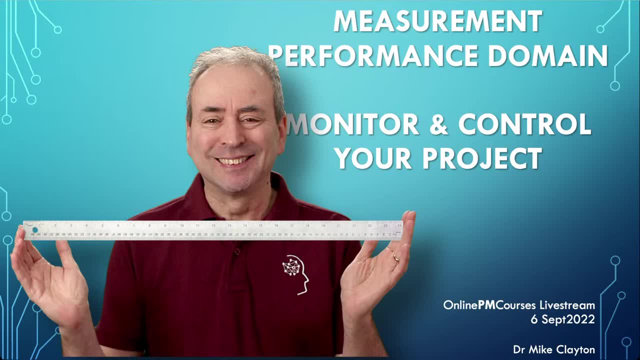 so yeah, i'm gonna talk about. one of the things i want to talk about is why i think the measurement domain uh is the best constructed domain uh of the eight in the pinbot guide. um, i've had some criticisms of others. i think this one's really good. i talk about the one thing i think. 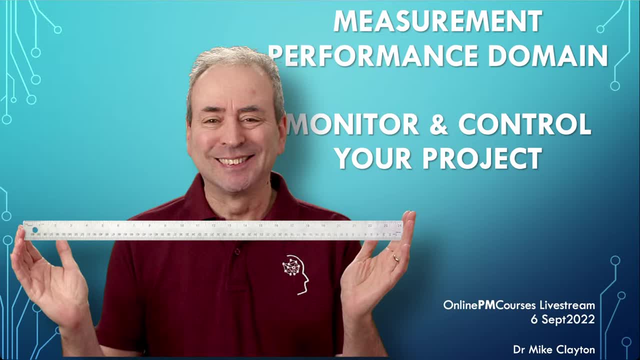 is missing, which i would like to see, uh, which i think would be really useful. um, and i think, i think measurement domain is the best place for it and, as always, i will give my five best tips. that relates to monitor and control and the measurement domain. i'll give you my two favorite. 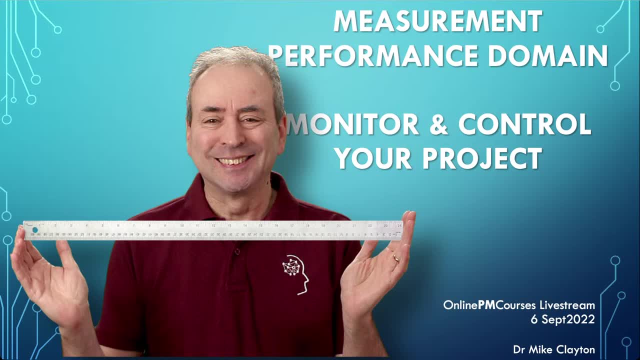 tools, um, for a measurement domain and my one primary insight. but what i think i'm going to do is go straight to the slides. keep. i'll keep an eye on the chat, but i'm not going to kind of keep putting my self on screen. i'm just going to flip back my monitor from how many people are in the stream, because that's. 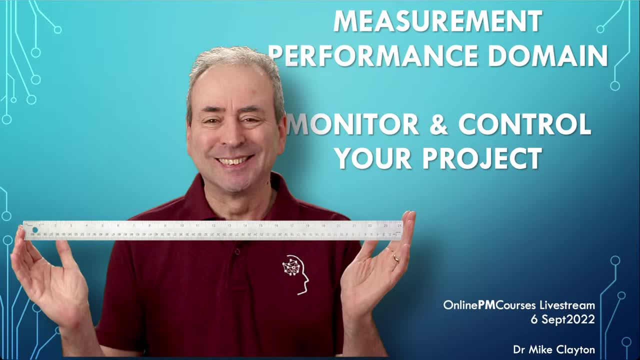 what's the word? i'm looking for vanity and look at the one thing that matters, which is the stream health page, and now it's reporting excellent, so i'm happy with that. it's great because this is where we get to the content bit. so, um, what uh? 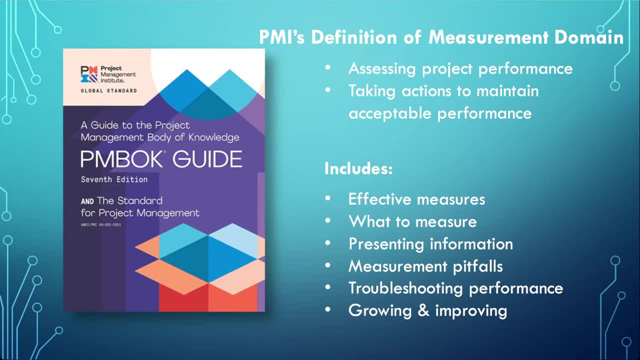 what we're looking at now is the measurement domain. this is the seventh of the eight performance. pmi defines it as being about assessing project performance and taking actions to maintain acceptable performance, and the sorts of things that the domain includes in the in the guide are effective measures to use. 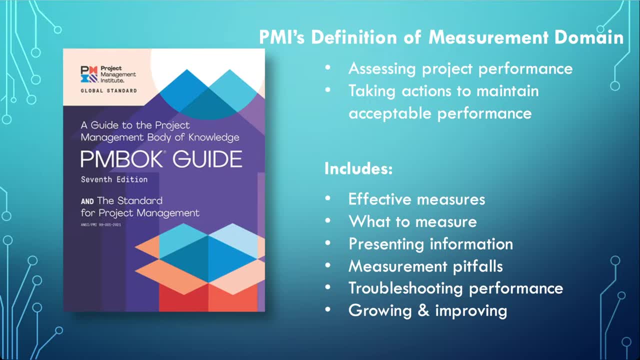 what to measure. i think they've got that the wrong way around, or maybe i just copied them the wrong way around. uh, presenting information, which is great because, uh, it does go a little bit beyond the fact you need to do a report- um, and talks about some of the tools you can use, which i like. 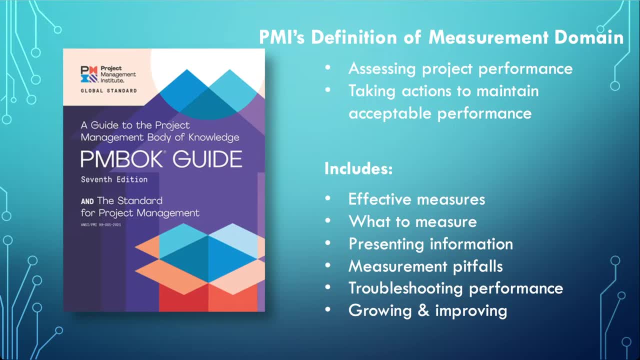 measurement pitfalls. now for me that's a a great sign of how good the um the section is, because previous pinbot guide basic guys to project management probably wouldn't have thought to include that and i think that's really nice section to have troubleshooting performance again likewise and then growing and improving. uh, so it's, it's got some really interesting stuff. 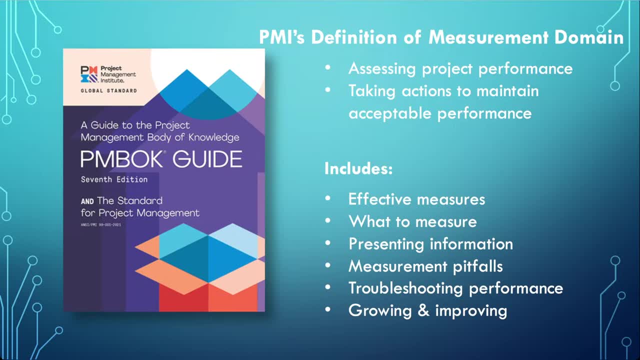 in it and if i, um, if i turn to that page in my copy of the pinbot guide, um, i'll have to turn to the wrong section. it's the next month's uh uncertainty domain. um, the, the measurement pitfalls- has some really nice ideas in there, things to be aware of. it's missing. 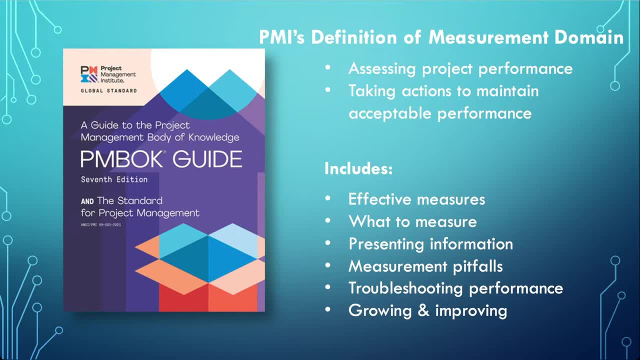 one thing i think, which i would have added, but, uh, you know, they can't thought of the hawthorne effect: the fact that, uh, when you measure people's performance, uh, the fact that you're taking an interest in them has sometimes have a bigger impact on their performance than the things you 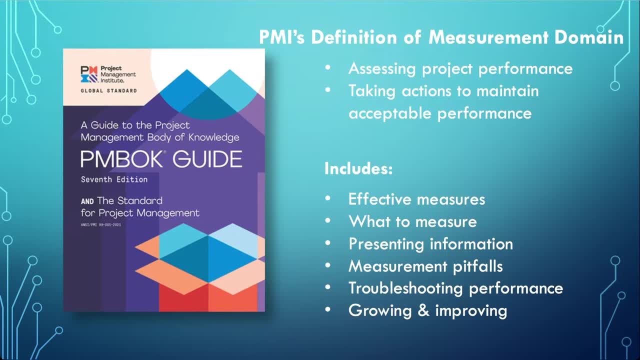 do to try to improve it, and i think it's important to think about how you can improve that. and now i'm going to turn to another subject, which is around, um, the uncertainty, and i'm going to talk a little bit about that, but first of all, i want to see how you can see more of yourself and the difference. 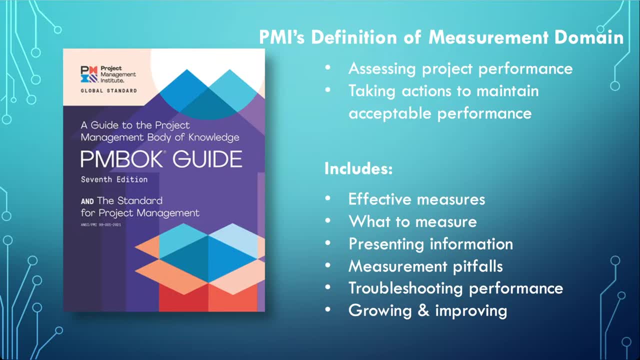 in which you see yourself and what you do, um more in what you're doing rather than maybe um the ambiguity- and i think that's quite interesting because that's uh pretty great. so, um, noticing what's actually going on- and we don't tend to notice things that go against our 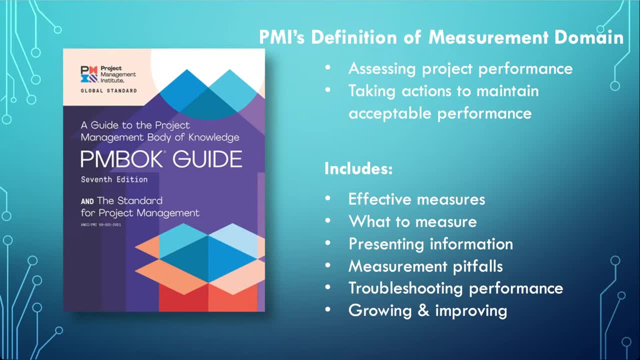 expectations? certainly not so much. of course, confirmation bias is responsible for a lot of the ills of human society in the world, because as soon as we have a prejudice, we notice things that endorse our prejudices and we don't notice so much things that conflict with them, and of 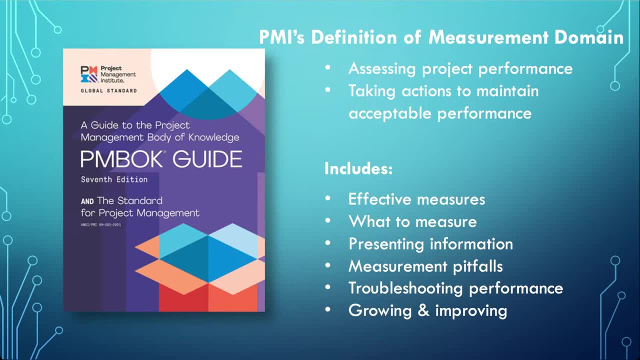 course, we all know that human beings have lots of inbuilt prejudices which we're not born with, but we acquire as we're growing up and it's very hard to shake them right. what have we got there? we've got to jessica, another new, another new name: jessica. hello from rwanda, great to see you, jessica. 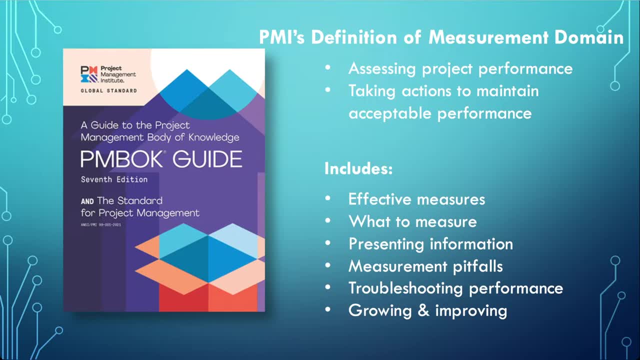 and abdulhamid. these performance interrelate with kpis. yes, in fact, one of the things that one of the things they talk about is kpis as performance measures, kpis, key performance indicators you can readily measure that indicate performance. now, interestingly, kpis are to some extent, 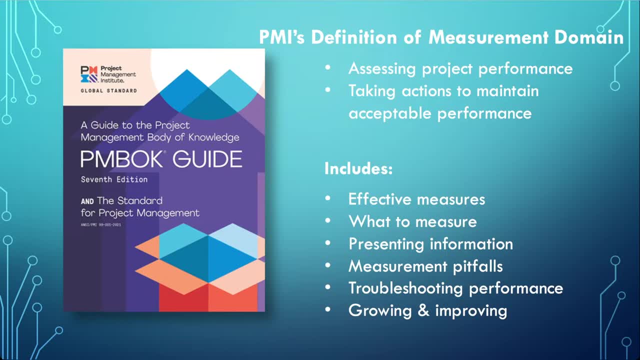 proxies for the things you want to measure it now. your ideal kpi will be a key performance indicator based on exactly what you want to know, but in the real world, quite often our kpis are a performance indicators that we believe represent a good proxy for what we want to know. and so what i would add to the list, the good list of six management. 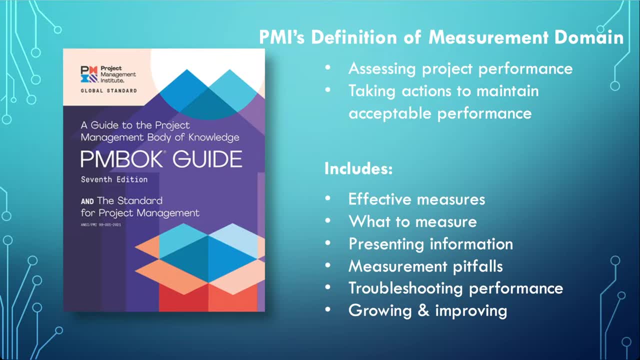 measurement pitfalls is proxies. proxies are a pitfall. you measure something that you think is related to what you want, but it's not a good relationship. it's related to misusing metrics, which they've listed. it's also related to the sixth one, which i didn't get to, which is correlation. 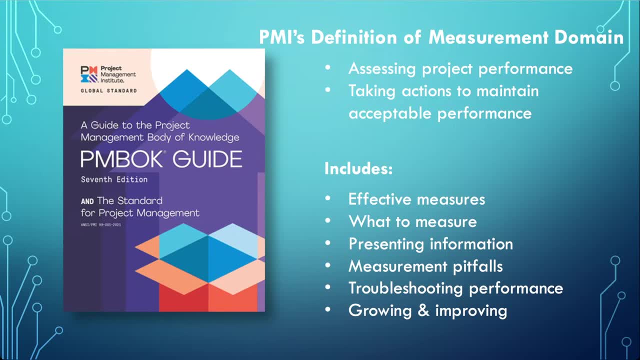 doesn't mean causation. two things that correlated don't necessarily have a causal link, which is true. two things can happen at the same time, but just because or or in a sequence. and it doesn't mean necessarily that just because one thing follows another, that it this. the one thing is because of 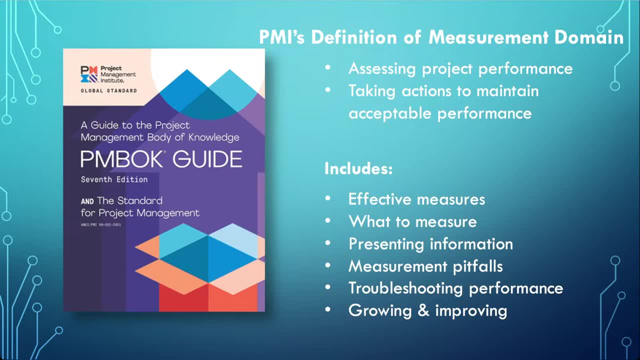 the other um, there's even a latin tag. what is it? uh pro, uh, post hoc, ergo propter hoc. after. therefore, because i do talk about uh kpis, uh, abdulhamid and um, and- and they do a reasonably good job of it- um, and then troubleshooting performance. they, they look at um using planned versus actual, um as a as. 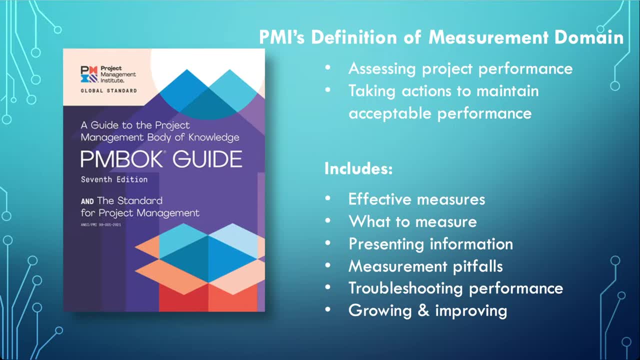 a guide example um an expenditure uh graph. um, i think probably, since they have earlier on talked about uh earned value management and earned value analysis, um, they could probably, uh probably should be relating it to earn value uh, more than just a simple thing. um, so it's a. 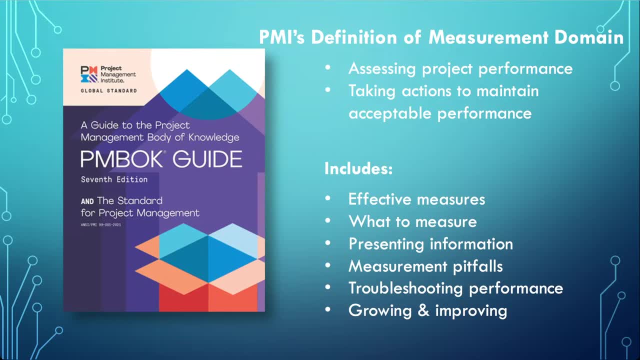 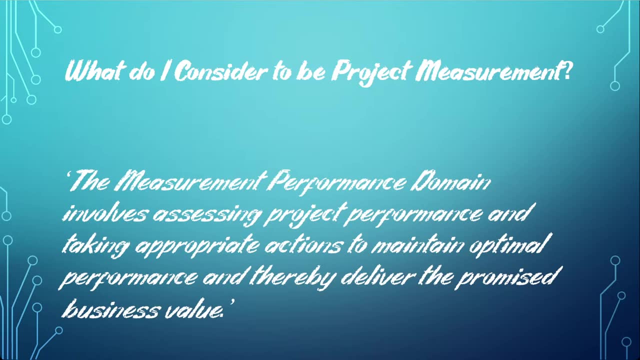 great it's, it's great it's a. there's lots in this and i really like it. so, um, uh, what do i? as as off as i often do, i i took a look at the definition and thought, well, it's good. uh, in fact, it is very good. 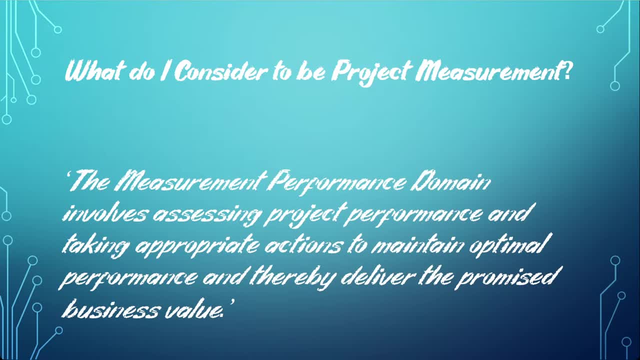 in fact, actually, if you go through, go through the first two or three pages of this performance domain, there is the definition, uh, which is the one that they quote. in fact, i can actually cite it for you. uh, they, they define the different measurement domain. um, it addresses, uh, the 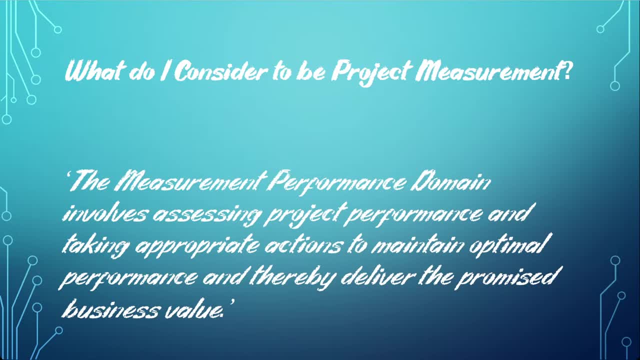 different measurement domain, um. it addresses activities and functions associated with assessing project performance and taking appropriate actions to maintain acceptable performance. but then they offer three alternatives, overlapping definitions in different ways. firstly, there's the: the list of the outcomes that you're expecting, uh, in the measurement performance domain. 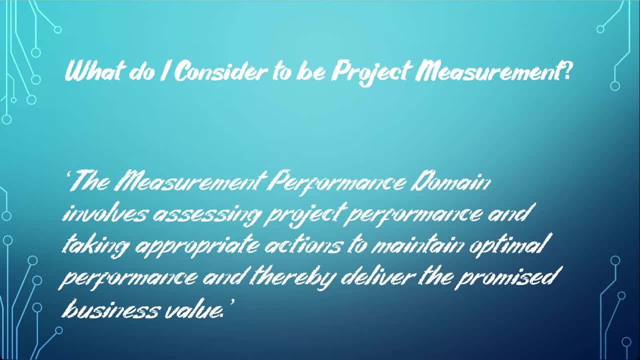 which provides another way of defining it. um then, then they just out and out. i like the reference to that is meeting the metrics identified in the planning performance domain. so what i like about that is, as a definition, is it ties together, uh, planning and delivery. and i suspect they didn't. 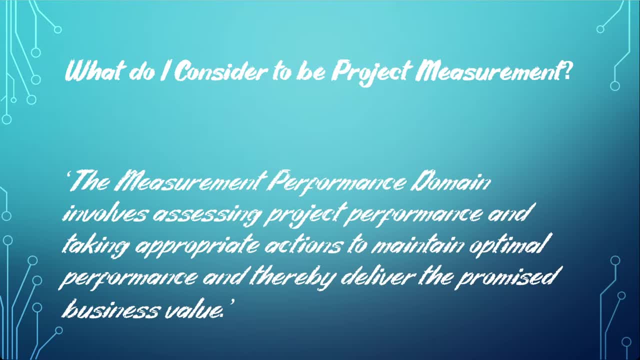 choose this as their formal definition simply because, um, that feels too much like it's about things, and i came up with my own version, which is what i consider project measurement to be. um, which is the measurement performance domain, involves assessing project performance and taking appropriate actions to maintain optimal performance and thereby deliver the promised business value. 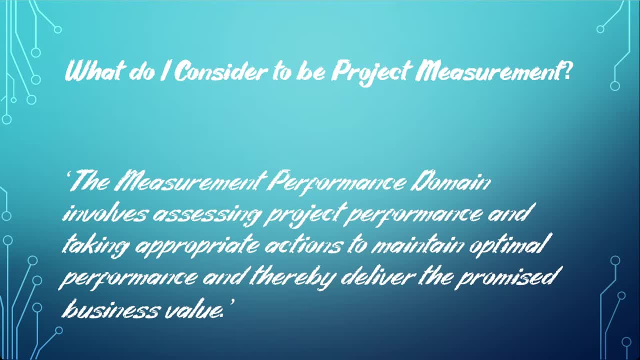 because they don't actually mention business value in this domain. and yet what are we doing, what? what are we doing? in delivering projects, we're delivering value for the business and uh, well, so so don't mention it. they don't talk about um, i don't talk, put it front and center, but actually, 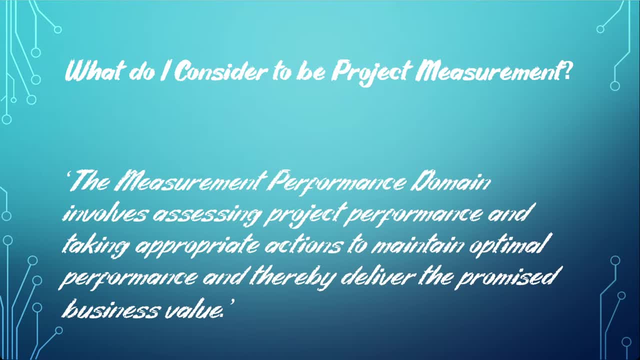 what they do do, which is really lovely. um is in section 2725, which is about business value. they have four different ways to measure value, which is great because they don't discuss it, uh, in comparison, but they do list four different methodologies: the cost benefit ratio, which is 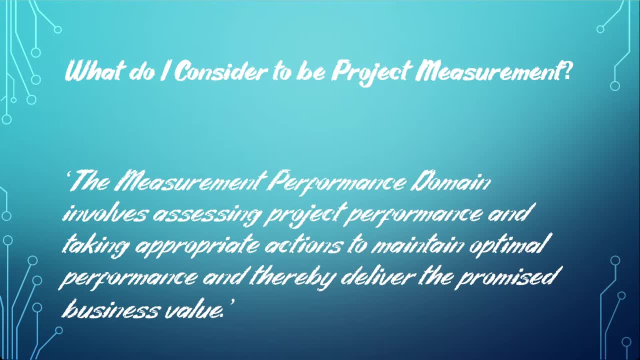 valued defined as benefit divided by cost. um, uh, planned benefits delivery compared to actual benefits delivery, which is quite nice. um, they don't use the, the approach taken by a lot of british project management organizations of saying, uh, value is the surplus of benefit over cost, which is value could benefit minus cost, which is a shame. but they do then go on to talk about. 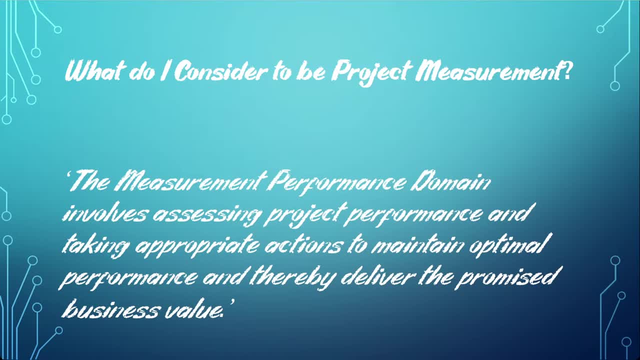 return on investment, which i think is the better measure, because it combines the diff, the ratios and the difference and it comes up with a nice formula. so the return on in investment as a value measure is benefit minus cost, all divided by cost. but then they also talk about net present value. i 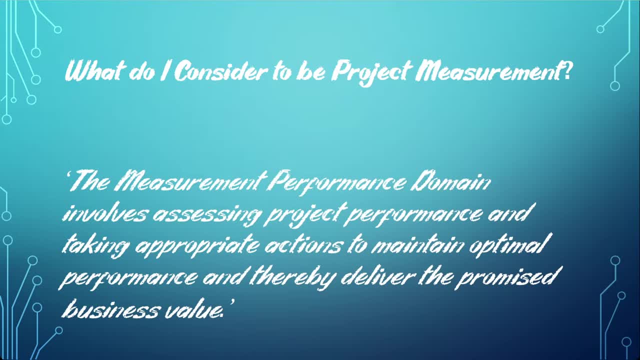 think the only place in the whole uh pinbot guide where they talk. when they do that, talk about net present value as a way to um measure value in a robust way, and i'll come back to that later. uh right, we've got a a couple of things. uh, i'm done checking five to ten minutes. 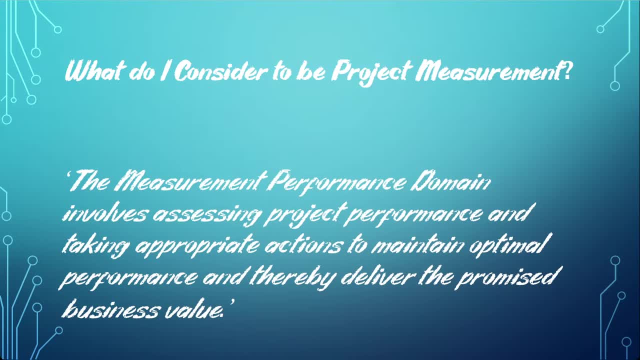 says hamburg gumbo. i hope that's not because we're all. uh, i didn't seem to. i still have a weak stream, but nobody's complaining about it, unless hamburg's just decided he can't be, uh, can't be bothered, which he's entitled to do. um abdulhamid says, and of. 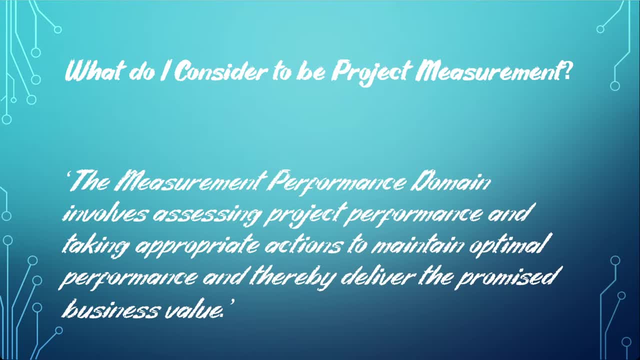 course, achieving high return on investment for the employer. yeah, absolutely. your whole purpose in delivering a project is to deliver the return on investment that they're expecting. that is the, the value to cost. uh, i'm gonna use a differential. it's a ratio, it's a difference. 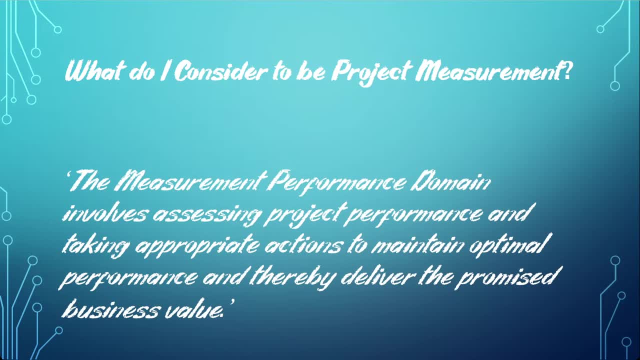 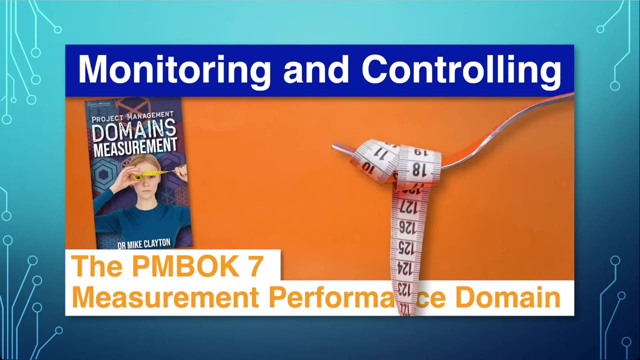 and i think the return on investment is a great measure. so i'm totally with you. so, um, so that's my definition: uh, bringing in business value, and uh, just as a reference, i have written a full article about this which is on my website. it went up on monday. come on, mouse. 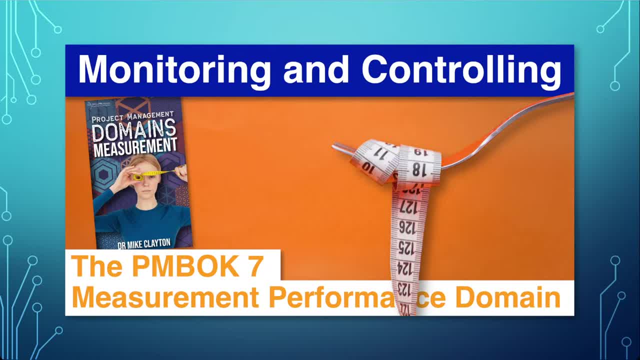 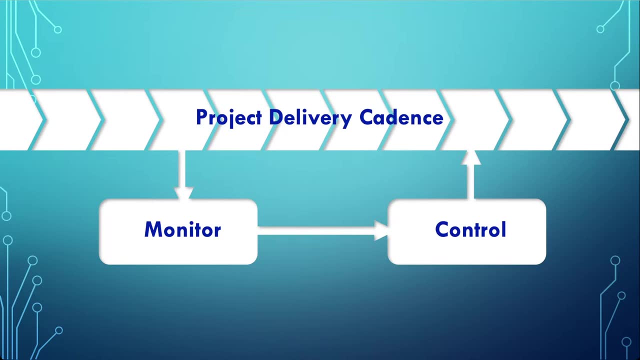 hop across. i'll post uh the link to that article into the chat just now and i have across the top. there we've got the project delivery cadence. effectively, the project is being delivered in whatever structure, whatever sequence, whatever pattern is appropriate to your projects. you've tailored your project uh to uh the needs and there may be a series of steps. it 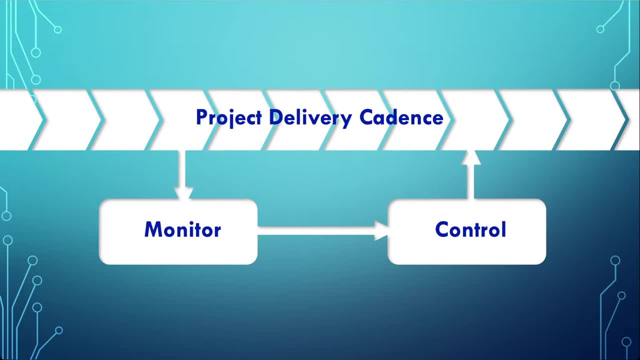 may be very continued. there are problems. i keep seeing red flashing lights on my dashboard. um fact, i am not sure whether you um, oh, i'm back to poor from no data, lagging, skipping, increasing, lost last 40 seconds. yeah, uh, all right, let's see what we can do. studio mode settings setting. let's push that down. 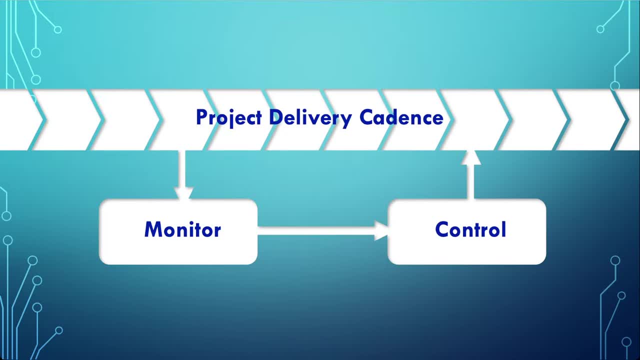 right down. okay, all right, right, i think i think i'm back. i think you might be able to hear me now. so i think we've got. we've got big problems with the internet. i'm gonna kind of struggle and see what happens. so my apologies to all of you who have taken 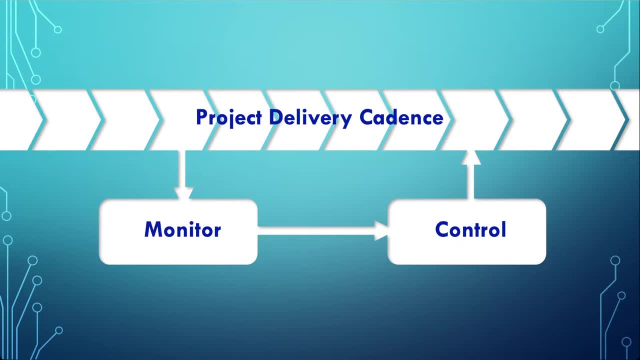 time to turn up um, um, yeah, when, when? in britain we tend to measure value as the difference between benefit and cost, whereas in the states i think you have to make it clear that, um, the, the value says more within the cost. elect cotton, silver, maybe on production taxes. but so yeah, i'd simply say that if you know it's something that's really important to consider- that you can do what you need. rest forged, it's possible, but if you can get it replaced, you might now be able to do it. that time, i think the time might be smart. another thing is going to matter after like: yeah, did you talk about studies, policies and 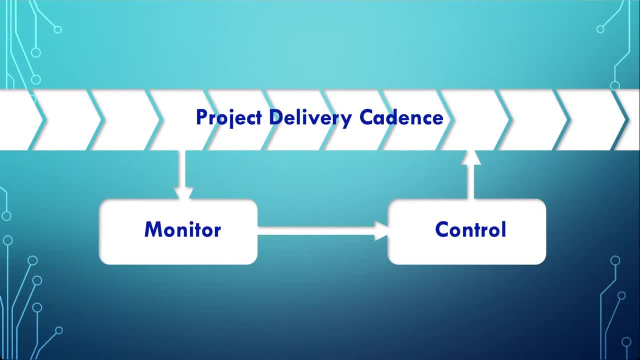 think the, the ratio of benefits and cost. um, so the numbers you get different, but you're still measuring the same things and that's why i like roi, because because finance people like it and finance people in the us and the uk and europe use roi. um uh right, so um project delivery cadence. 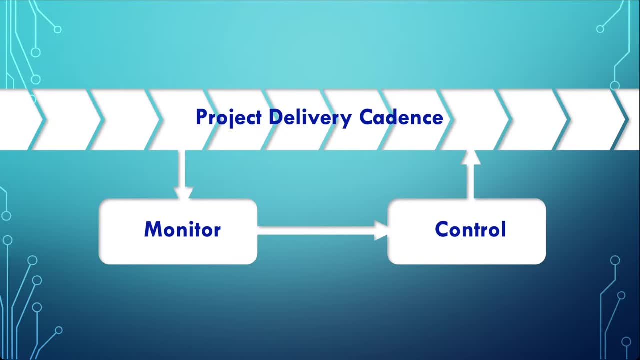 uh, what we've got here is projects being delivered periodically. you monitor. the primary reason why we monitor our projects is quite simply to find out if there are problems and then we can take action to restore control, because, as project managers, the thing we crave above all else is control. 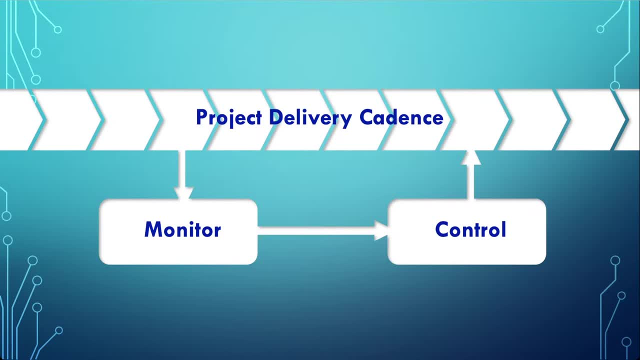 youtube is continually telling me: you're having a bad experience, but there's nothing i can do about it. this is really annoying. this is really, really, really upsetting. i prepared this carefully and it's just throwing me through. um, okay, i'm going to keep going. so here's. here's the thing. um, what we try to do is we try to monitor and control within the kind. 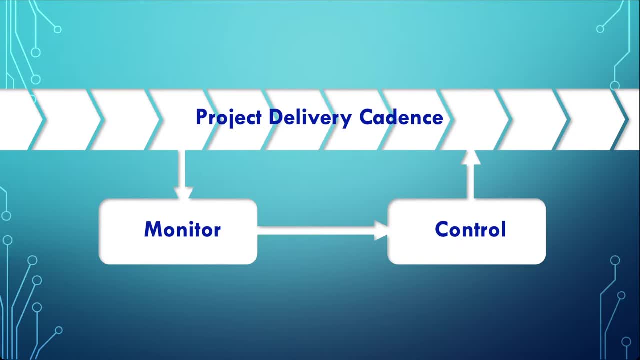 of delivery cadence, that is to say, if we're producing stuff everywhere every day, we need to monitor and control every day. otherwise, if we wait too long, then by the time we spot problems, those, those problems have escalated and the controls we would need, even if we could make them um, are significant. if, on the other hand, we spot our problems early, then 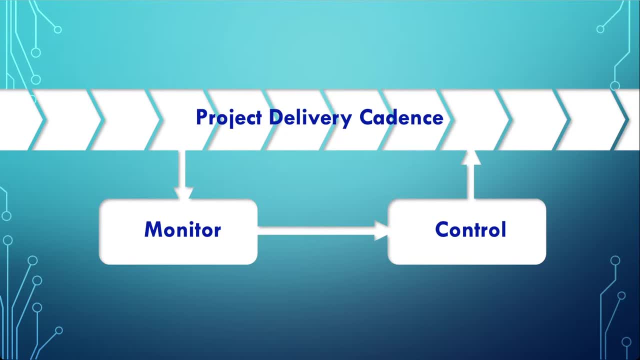 the controls can be subtle and easy to do and if we're monitoring frequently enough, we can see check very quickly if, uh, our control is not as good as it used to be. and if we're monitoring as 저으 funnel not completed, the controls have worked. 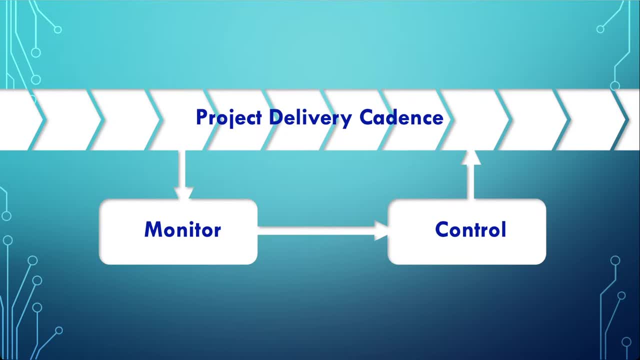 if you drive, or if- but it's slightly less uh uh evident if you cycle. if you're driving or cycling down a long straight road, um, although you think that you're holding the steering wheel or the handlebar steady, what you're actually doing is adjusting them a thousand times a minute. just tidy. 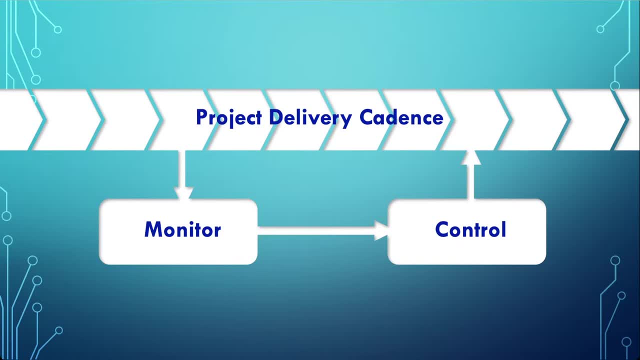 tiny tweaks to keep the vehicle going straight, visible in your motion, if you deliberately did hold it dead still and wait to newspaper behind you to check where it was. the engine was knocked off and about ten minutes later something stopped by and the pulled down a little bit. 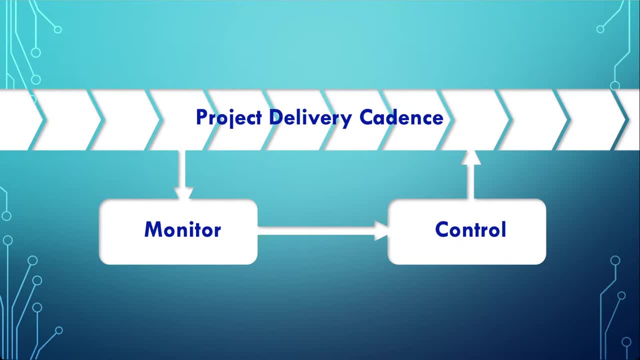 approxオ till you can see that you're starting to swerve, then your body would make a correction, but chances are, unless you were very skilled, you'd over correct and then you would have to swing back and you get into an oscillation and quite literally it is quite possible, because it does happen on 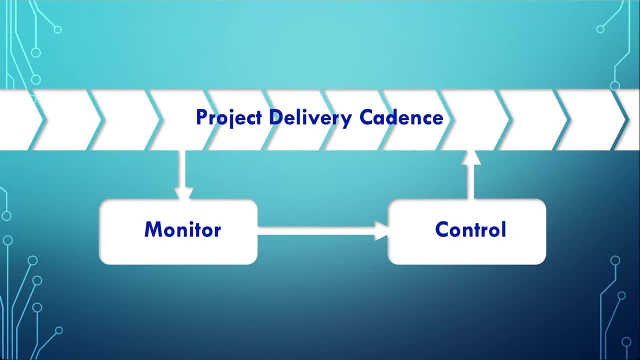 motorways, particularly when people fall asleep on the wheel, that you can spin out of control and projects are just the same. if you wait too long before trying to correct your path, then your project will spin out of control. so what matters most is the monitoring. control loop has to be. 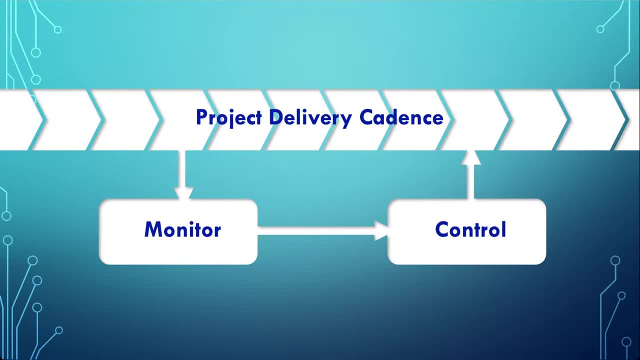 fast enough now. a classic example of this in the modern world is scrum projects, which have daily stand-up, daily project stand-ups and those scrum stand-ups- scrum stand-ups- are the ones that you can do the most of the time. you can do the most of the time. 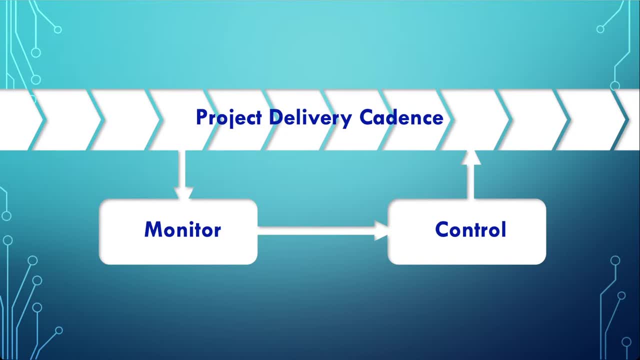 scrum stand-ups are the ones that you can do the most of the time. you can do the most of the time. scrum meetings, whatever- are a great way to monitor what's going on and for the team to apply control. but you say, hang on a moment. does that mean the fastest cycle time you can have in? 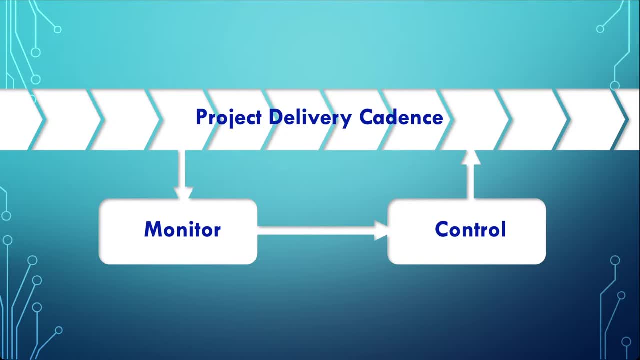 a scrum project in an agile project is daily, but surely the team are changing code much more frequently than that. there are plenty of changes during the day. what happens if things go wrong? well, actually, this is is where test-driven development was created, the idea that you. 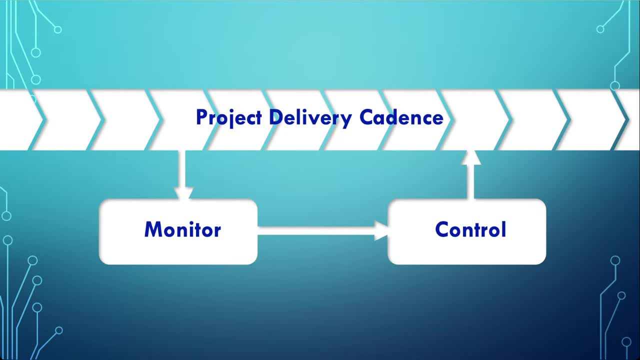 start your development process by defining the tests and then pretty much every change you make, before you commit it, you actually test it and see what happens, and if it doesn't pass the test, you figure out why not put it right and wait till you get a positive test before you start changing. 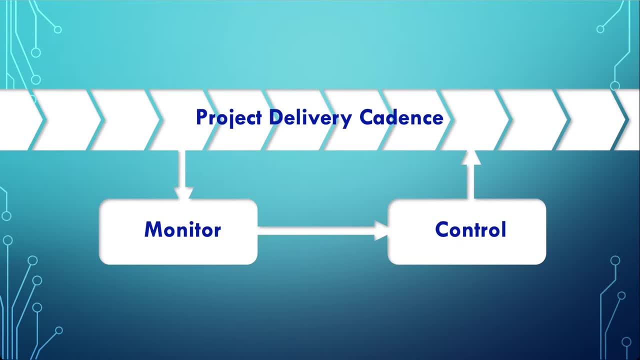 anything else. and what that effectively does is it puts in a monitor and control loop that's going to control loop at the developer's desk, at the developer's monitor, literally every five, ten, fifteen minutes, sometimes even even faster than that penny, so we can monitor control almost at the speed of 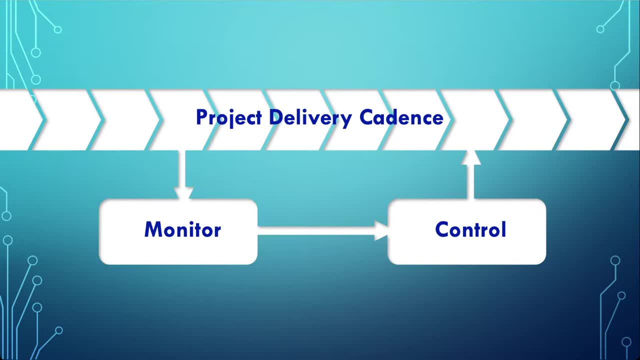 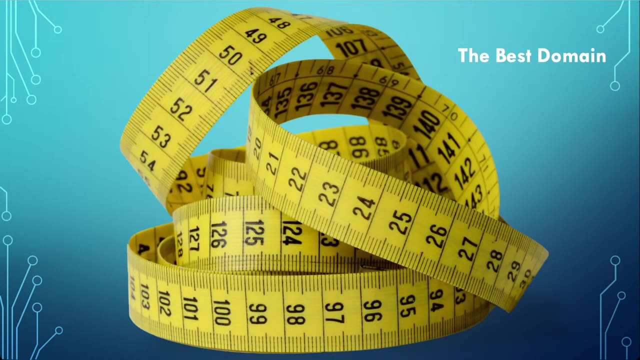 thought, and so that monitor control cycle I think of as the beating heart of the project during the delivery stage, and I do think this is the best domain in terms of it's not. you know, I wouldn't have been my favorite domain if I, if you just said to me: oh look, here's the eight domains, Mike, we know what. 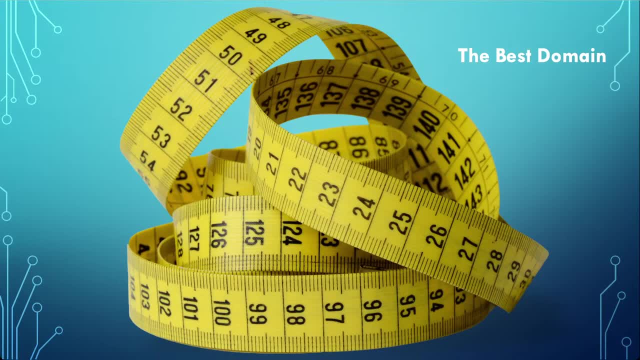 the eight domains are gonna be. they're gonna be stakeholders, they could be team development, approach and life cycle. they're gonna be planning, project work, delivery, measurement and uncertainty. so there's your eight performance domains: which, which, which, which will be your favorite? I mean you. you would probably, in fact, if you can hear this, 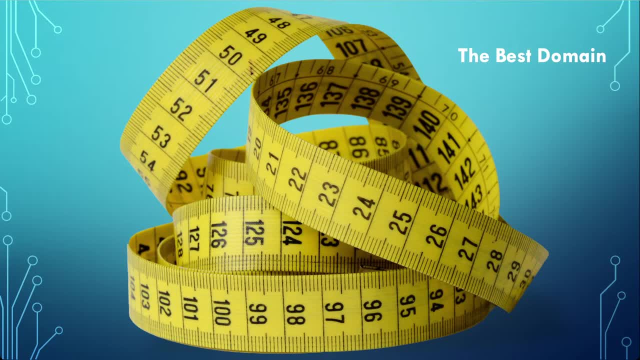 put your favorite topic of those into the, into the chat. I suppose my favorite will probably be the stakeholders or uncertainty, because those are the ones I've spent most time thinking about over the years. that's the one I've enjoyed and learned a lot about, but my favorite. if I'm assessing what 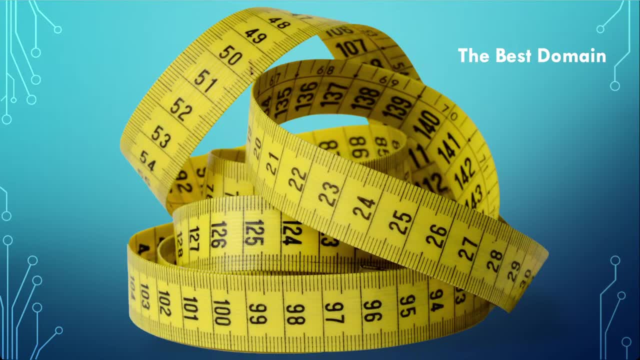 has been produced by the pin book seven development team, which one do I think they've done the best job on, is Azure, absolutely, absolutely the measurement performance domain. and and the reason I think it's because, firstly, it has strong definition of domain. it has some strong definitions within its of elements of 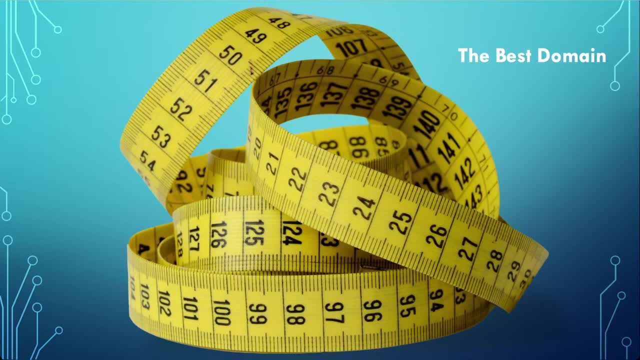 the domain, which which work really well there. the definitions of metric baseline myself you haven't all dropped off, no, you're still there, that's great. so yeah, in the uncertain performance domain, is a is a? there are some pretty rotten, ropey, old definitions, and, and I don't just mean I don't like them ». 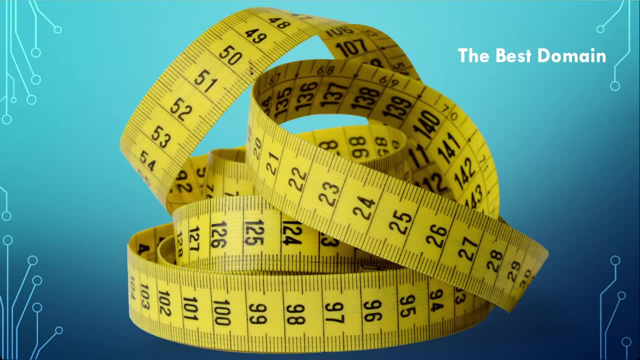 think some of them are wrong. I think the poor definitions that are emerging on, and possibly even absolutely, in an absolute sense, wrong, yeah, in fact. in fact, the definition of ambiguity is just not right. it is wrong. measurements domain, though that that's the It. government's are great. 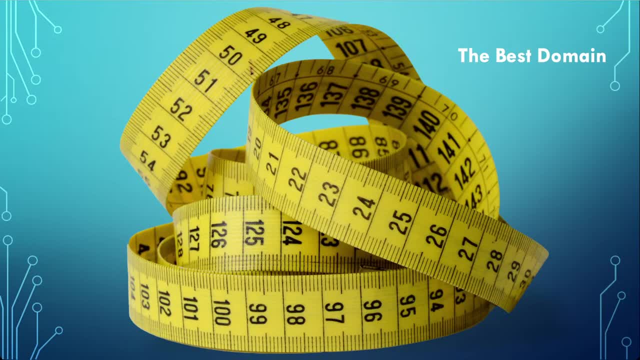 I think the one definition and let us seen in their dance listed is it's forecasting performance value, probability, and it basically is pieced teams and then the people with the higher and girls for every feature and I think, some common definition into the world. we said as well. basically, and this is probably one of the fifest, 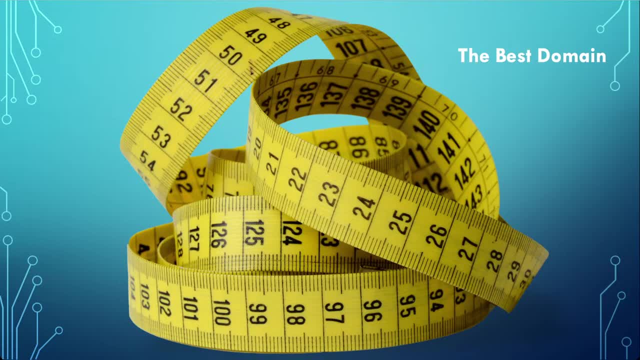 because they talk about baseline. um, we talk, the whole thing is about measurement and i'd like to see forecast defined there and i define it in my article. so it's great. um definitions. the domain has great coverage of its topic. uh, if you take its definition of what the domain is, 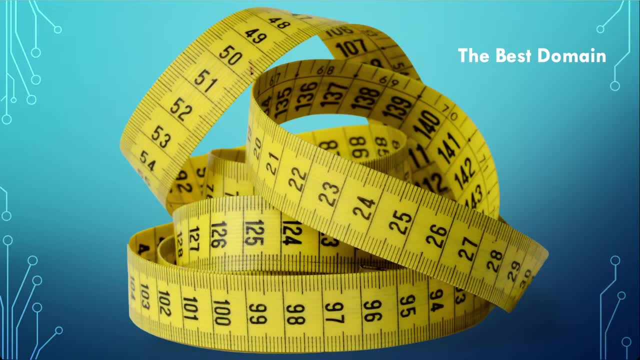 i think it is very nearly complete in its breadth. it is good in its depth. they get the right balance and the information is really, really nice. there are some lovely elements. there's plenty to think about what they talk about. they talk about well. they talk very clearly and precisely and usefully. 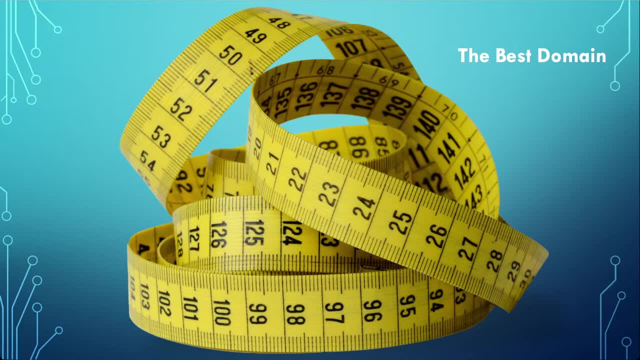 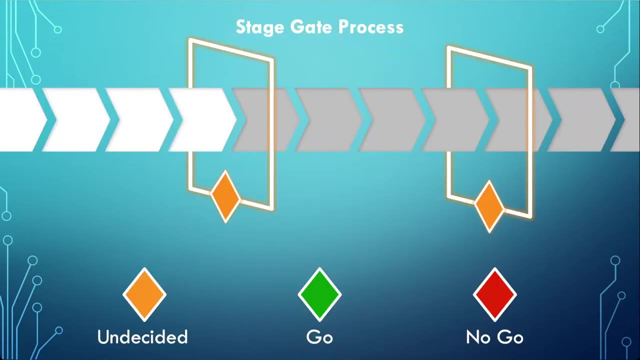 and thought-provokingly, and it is very strong in the sense that they set out to write a pinbot guide which is heavy on principles rather than on practice and domain is the stage gate process. the stage gate process is, and i think it belongs, in measurement, but i could 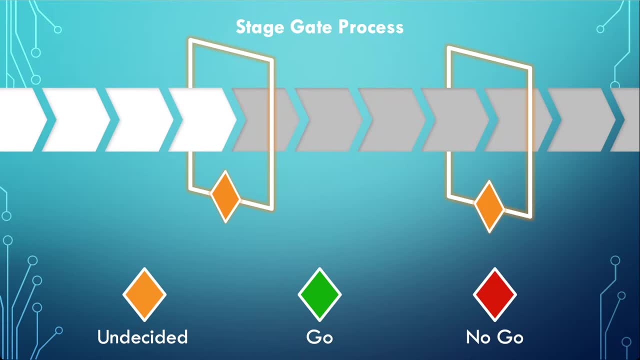 you know i could take an argument that it should live in life cycle, but i should check- i didn't. i forgot to check at the time i wrote my review of it- um, whether actually it does appear in life cycle, which would be a sensible place to put it, but it's not necessarily where i would put it, um. 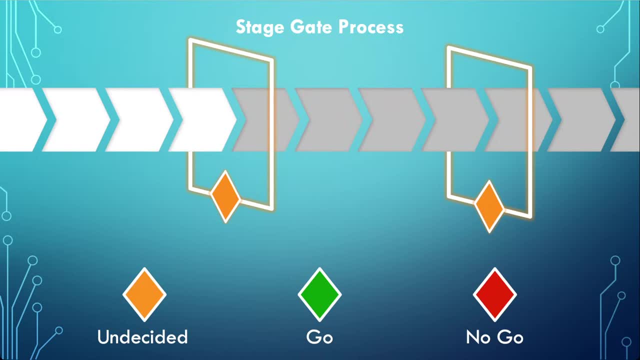 hang on. let's have a look at the life cycle planning navigating way through this right performance. development has development approaches, considerations and selecting the development approach, life cycle, phase definitions, aligning delivery cadence, development applications, interactions with no, so the development approach and life cycle doesn't. 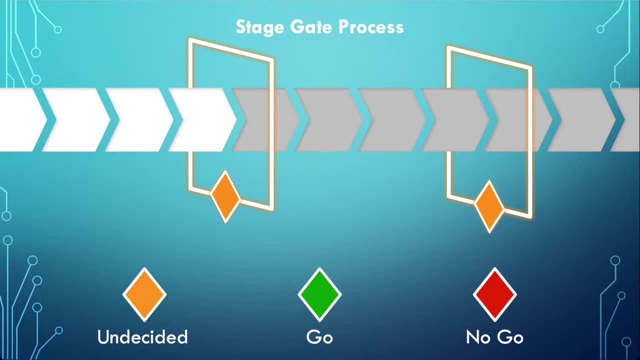 have a stage gate process as well. now you could argue that if agile projects don't have stage gates and therefore it doesn't belong in pinbot guide- because pinbot guide is now um agnostic around predictive versus agile, so anything that is peculiar to one shouldn't be in there. but actually you could argue that um sprint reviews. 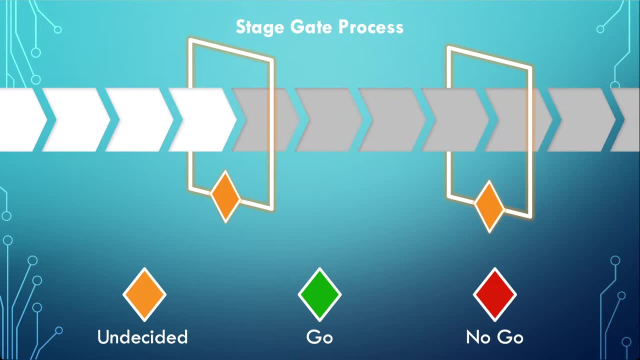 are stage gates. you could argue that the decision, the sprint planning process, the decision to draw more user stories down into a sprint backlog and and have another sprint is a stage gate determining whether there is benefit, there is value, sufficient value in further work. so yes, i think agile process has stage gates. so what is the stage gate outside of the project? um, for kind of. 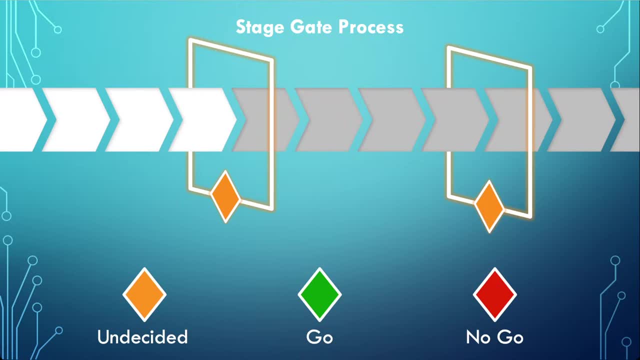 low stakes projects it's probably your steering group or your project board or your governance body. uh, for very high stakes project projects it's going to be a group of people from outside of the project entirely, possibly even outside of the organization, have uh stage gate processes run by. 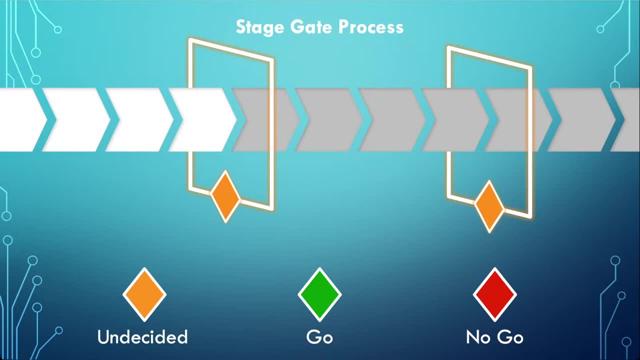 people from other government Department and also outside of government entirely. so those people will review where the project is at the time. they will assess whether the project team understand the status of the project and have. they will consider the level of risk that the project propose offerers and as long as they meet a Dec regulation. 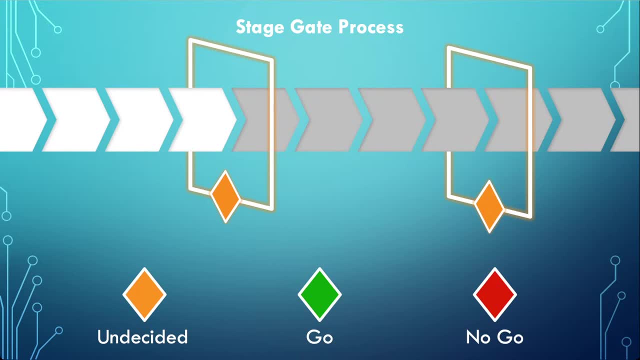 As a result, they will make a go-no-go decision, and if they make a no-go decision, the project will stop and there will be no more funding. If they make a go decision, possibly subject to caveats, the project can then continue. 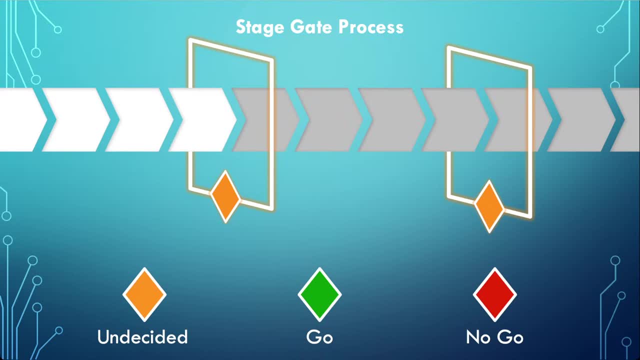 and draw down the next tranche of money, And so the project then proceeds to the next kind of stage or phase whatever. So we set up a series of stage gates, usually sort of three, four, five stage gates. But you can apply the principle to add control, accountability and governance to any project. 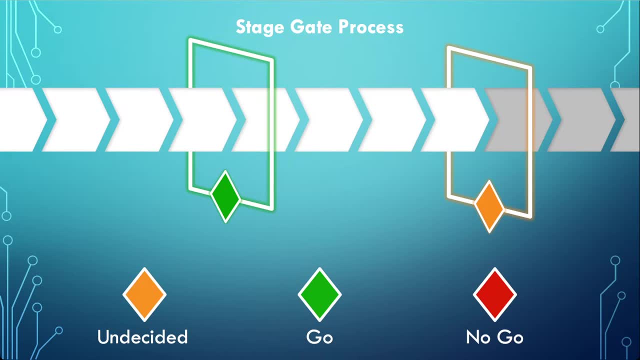 And I think this is such a powerful approach to ensuring you get value for money, ensuring you contain your risk. Gateway review process is taking off. So let's get on to my three. two: one for project delivery. Oh, it says project delivery. 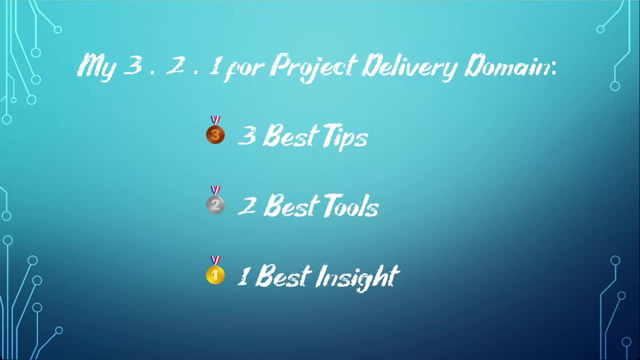 It should say project measurement domain, My apologies. So for the project measurement domain, three best we often talk about. well, in fact, what we often talk about, that's the wrong way to introduce. seven offers us effective metrics and it suggests that they need to be smart. 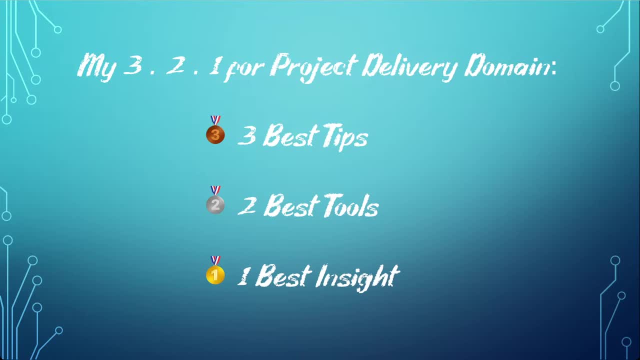 And it defines smart as specific, meaningful, achievable, relevant and timely, which is spot on. They also then go on to say the smart acronym can use alternative terms. For example, some people prefer measurable instead of meaningful, agreed instead of achievable. 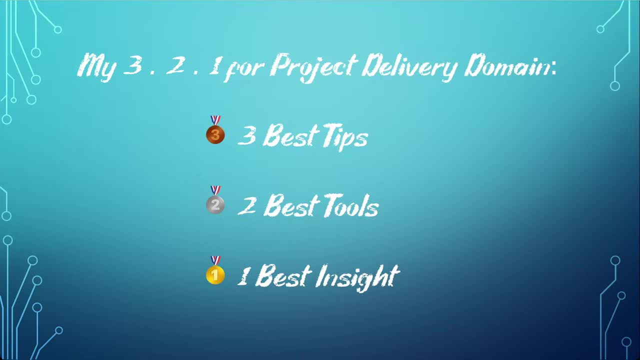 realistic. Going to suggest that you do is actually take an even wider view of smart. So let's just have a look at what some of the alternatives are that go beyond the ones they've done. For a start, I don't like using specific and measurable, which is one of the commonest. 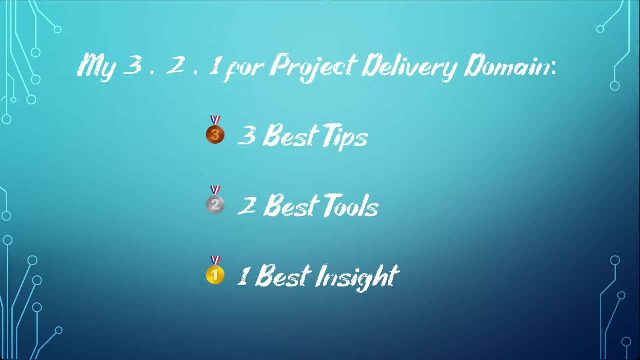 ones because I think measurable. if something's measurable, it is pretty specific. So I like the fact they've gone for specific and meaningful, but you could replace specific with stated and then have them measurable as well. The A can stand for a lot of things. 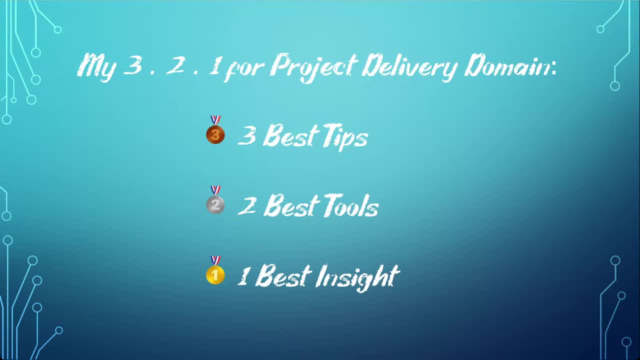 They've suggested achievable or agreeable. So let's look at that. They've suggested achievable or agreed. Actually, do they Yes Or agreed to? And I like agreed as well. I also like the possibility of having them as aligned- aligned to what we're trying to. 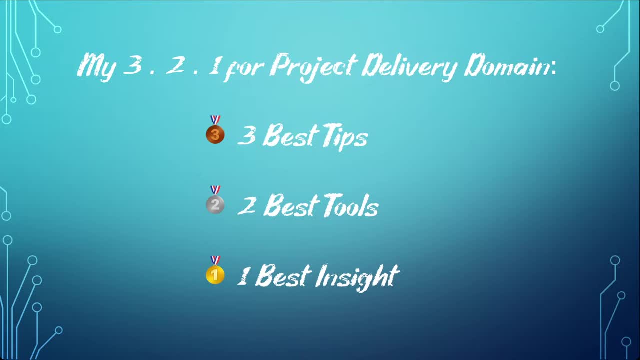 achieve, And there's quite a nice alternative version of smart, which is shared, managed, aligned, responsible and tracked, Which is completely different. What I like about it is it's completely different to the standard ones The R could stand for: realistic and relevant, but also rewarding. 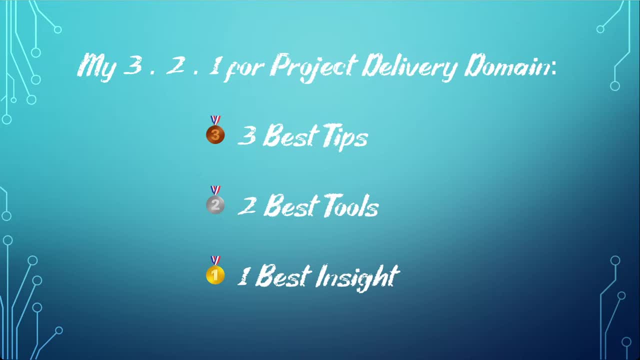 I quite like that one as well- Or responsible, And then we've got the T could be timed, of course, or time bound, Tracked, tested, or testable as well. OK, Great, Thank you. And then, of course, you can extend the smart framework to make it smarter where the E. 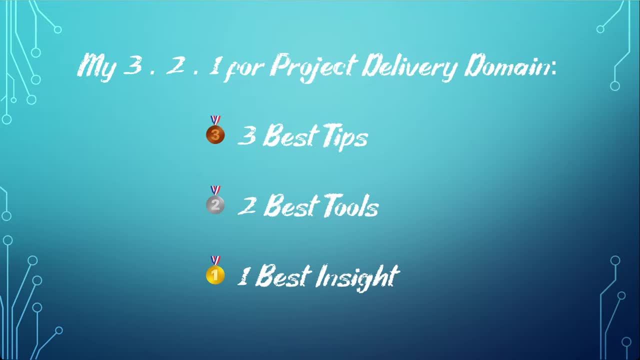 could be ethical or ecological, or even exciting, And that allows you to use a second R, which could be something like recorded or reviewed, as well as rewarding or relevant. Indeed, you could even go for smartest and reuse another one of your S's. 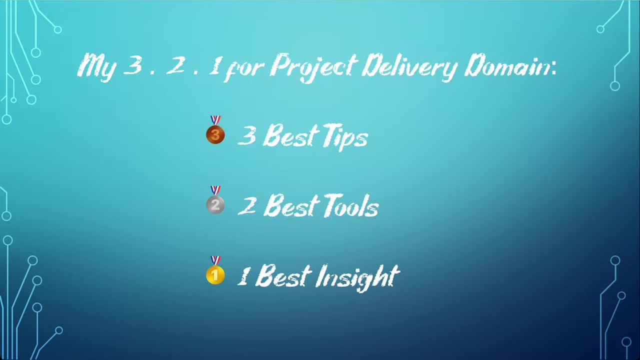 And another one of your S's And another one of your T's. So my first tip is to go with a, to draw from a wider selection of words in your smart acronym, which they wisely suggest. The second is to call back to Peter Drucker. 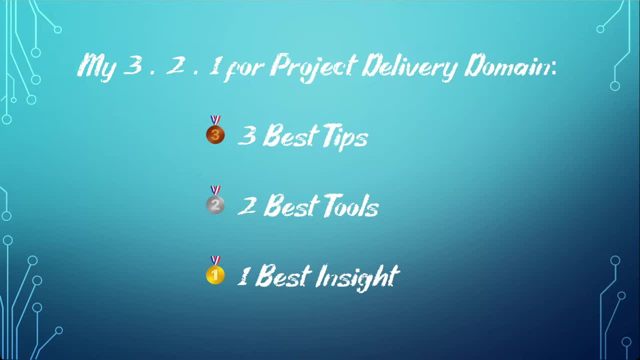 Peter Drucker, a famous management thinker, said: what gets measured gets managed, Which is exactly why we measure in our projects To help us manage things. But what he was pointing out is that if we don't measure something, we can't manage it. 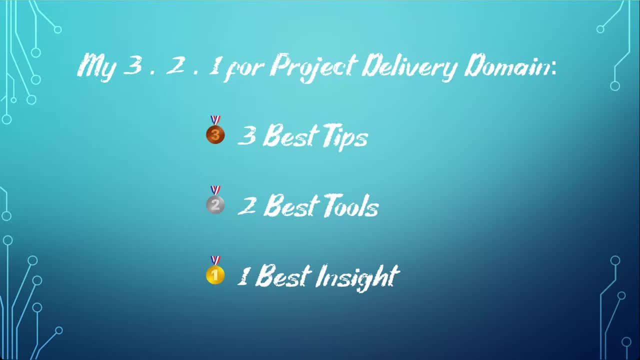 So we tend to focus our management behaviours on the things that we measure, And that is another call to make sure you measure the right things. And when I start a project and periodically through the project, one of the most important things I do is I consider what are my big levers. 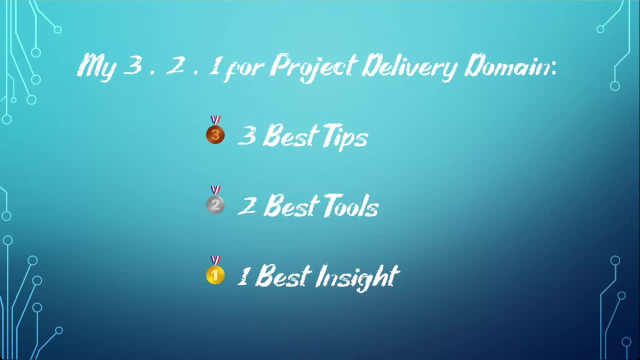 What are the things that I need to pay most attention to, because these are going to be powerfully influential in the success or not of my project? It may be risk profiles, It may be quality of deliverables, It may be schedule performance, It might be resource allocation. 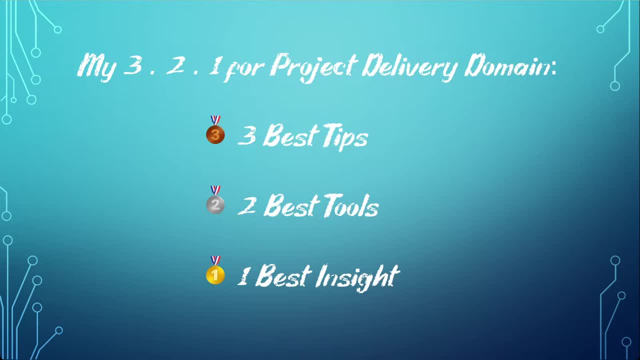 It might be capability of resources. Usually there are one or two really big levers that you can pull which will have a disproportionate effect on the outcome, And then obviously we need to measure those. So that's my second tip, And my third tip is just to fill in that kind of warning that isn't in. 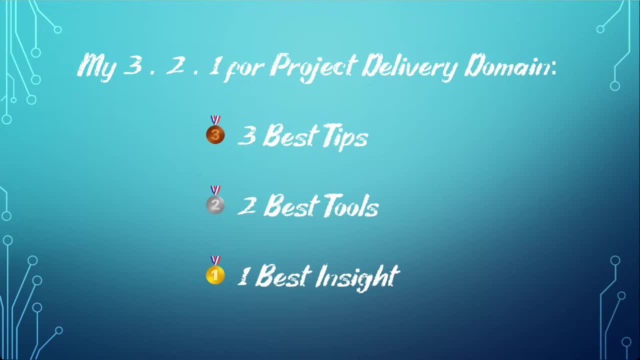 Pinbox 7,, which is to take care of discount factors, And if you are not familiar with discounted cash flow method, I have an introductory video on discounted cash flows which is well worth taking a look at And if I get a lot of good feedback on that, 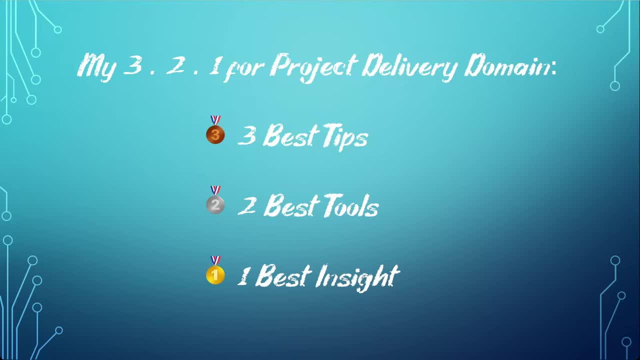 it's an old video but if people kind of really want it, I could perhaps make a more detailed discounted cash flow video Or article explaining the process. But what discounted cash flows do is it basically looks not just at the total costs and the total benefits but the timing of each piece of expenditure. 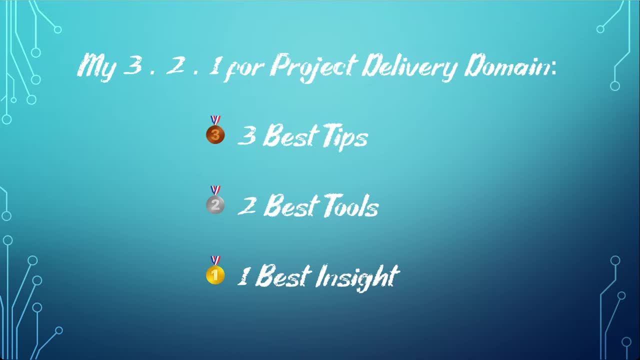 of each receipt of benefit. And, of course, it recognises that timing matters, because if I offer to give you $1,000 in two years' time, that $1,000 would be worth a lot less than if I offered to give you $1,000. 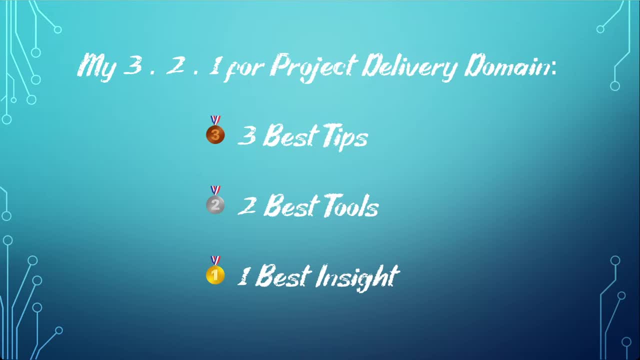 Now because inflation would erode its value, whereas if I gave you $1,000 now, you could put it in the bank or you could invest it and potentially it would be worth more than $1,000 in the future. Now getting your head around inflation rates and performance. 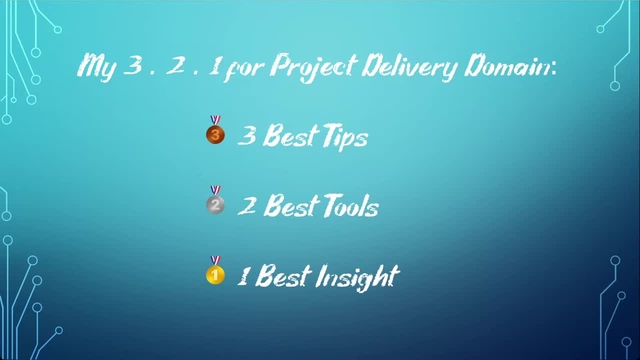 my favourite tool to visualise performance and progress and status is a Kanban board. I absolutely love using Kanban boards. They are great for many different sorts of projects. There are, of course, many. There are many projects for which they're not appropriate. 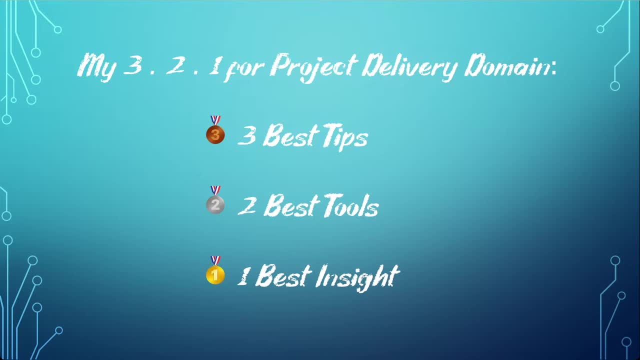 I understand that And there are many tools that you can use to create them. I think Microsoft Suite has a Kanban board. Asana, Jira Monday. all of those three tools are on the website a while ago And, of course, my favourite is Trello, which is standalone and has a fantastic free tier. 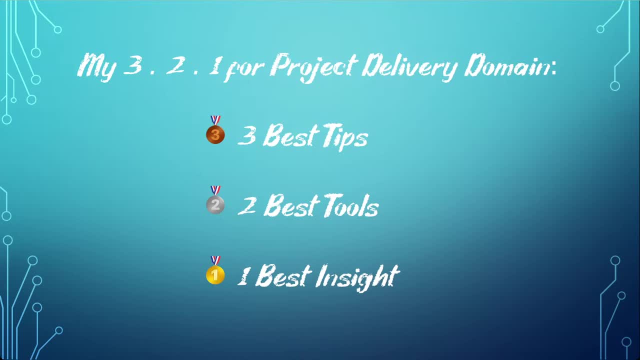 which means just the right KPIs for that project And crafting those KPIs and finding proxy KPIs where you can't measure what you really want to measure. it's a lot of work. It's very difficult. One of the very early projects I did. 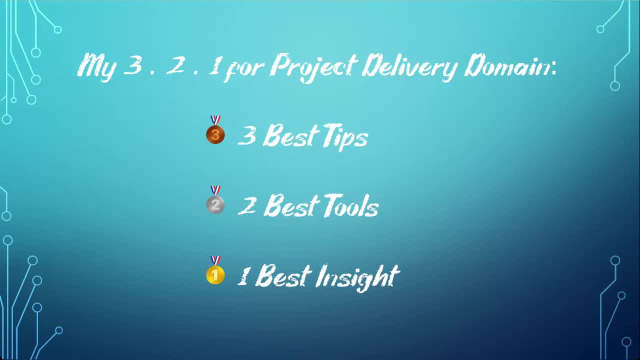 I really understood what matters in a good housing service in the British local government or English local government arena And interestingly I still have a client, a different one, that is a London Borough housing team delivering different services to them. I think now I did that under guidance at the start of my career. 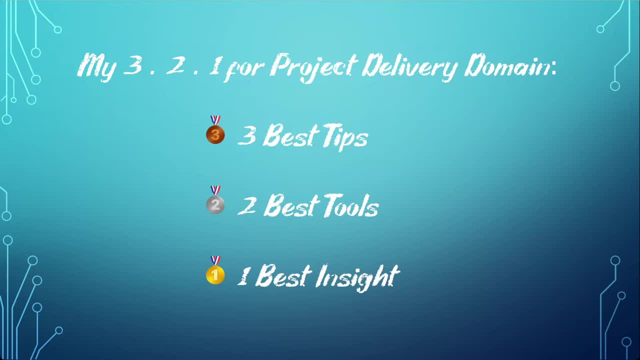 I'm not sure I have the skill to do it again now. So those are my three best tips and my two best tools. What's my one major insight? It is really to monitor within the cycle time, the natural cycle time of your project. 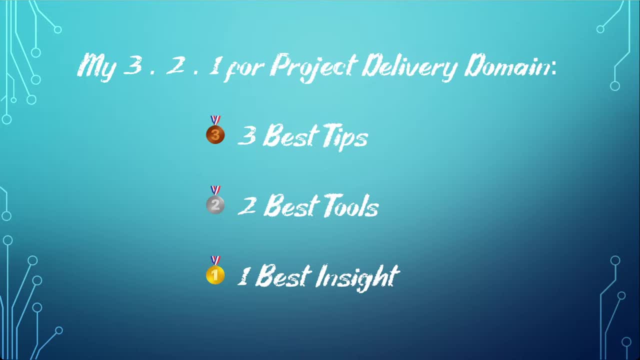 You know the pace of your project because you know that you have worked on projects where nothing much happens from one week to the next And therefore you don't need to be measuring what's going on and monitoring what's going on every day, because nothing will change from day to day. 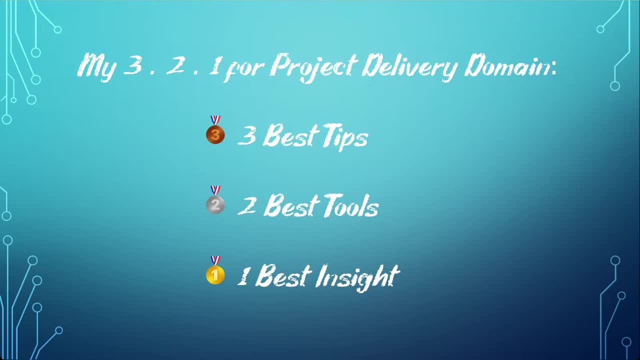 You've probably also worked on projects where actually, if you step out for a day, then things have changed And therefore you do need to be monitoring every day two, three, four times a day, And if you understand the cycle time of your project. 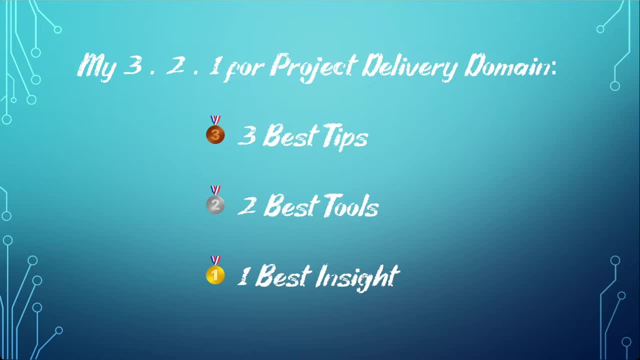 then you will understand the appropriate kind of monitoring regime And it's also why I believe there's the no, it wasn't Hillingdon. You need to make sure you have arrangements with a suitable colleague to act as your deputy, as project manager. 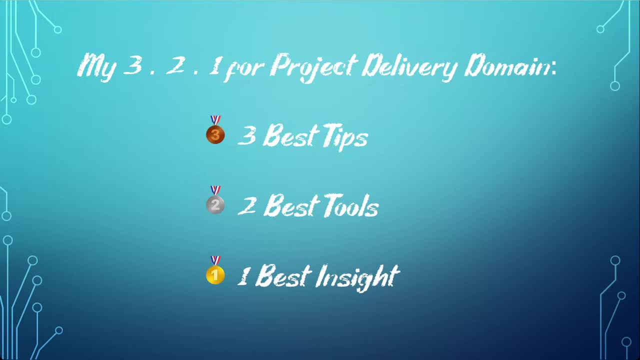 because someone needs to be managing the project at all times. It was a. there was a TV program on British television about, I guess, 5,, 10,, 10, where a celeb was trying to renovate a big old house. 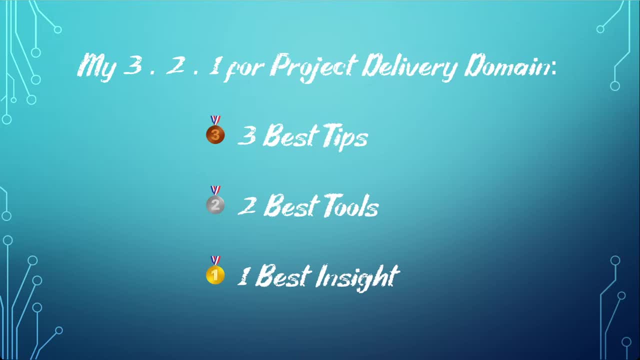 And she was doing the project management Monthly she had to travel up from her home in south of England to her project renovation building in the north of England As she came up with the family once once a full and she had during that weekend to balance the family and her young children. 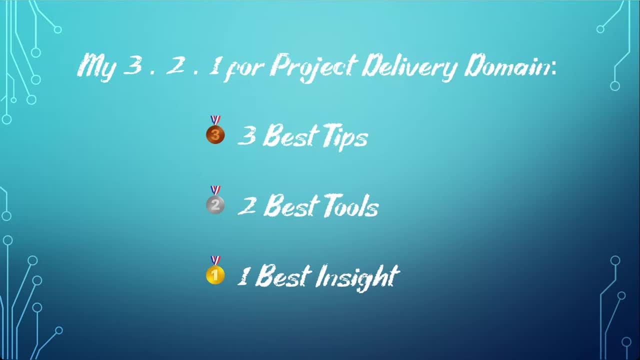 and managing the project when pretty much all the tradesmen and contractors and consultants were not on site, because it was the weekend and the project was failing massively. because she was trying to be an absentee project manager and she wasn't managing the project and it wasn't working. 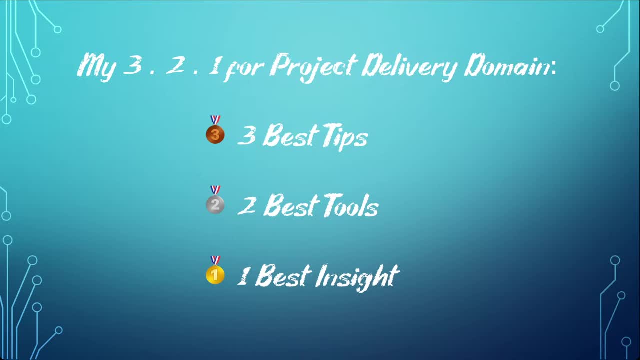 We're professionals, We don't work like that, but that's just kind of my take on things. So where are we still seeing? lots and lots of problems with the stream, And I'm so I can. all I can do is apologize again. 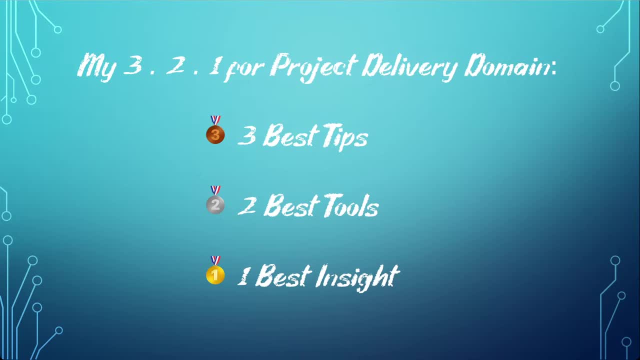 Hope you can hear my apology First. I've got a red light So you probably can't hear my apology, but I'm going to say it anyway. Streams not performing Well and I apologize. Domains: each e-book contains my review of the domain. 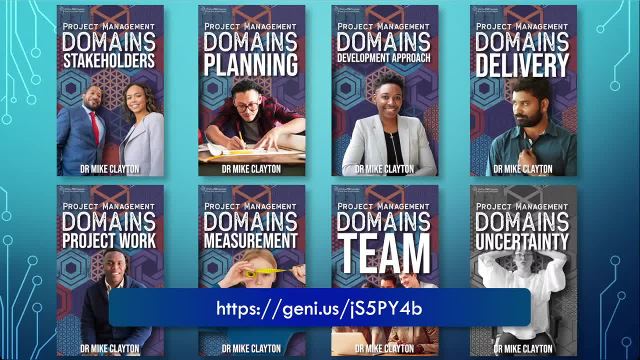 my review of the domain principle, the kind of idea of project management domains in the pinball guide, my review of the specific domain We're talking about, and then a number of articles gathered together to explain in depth that domain, and there's a lot more content in those e-books than there is in pinball guide. 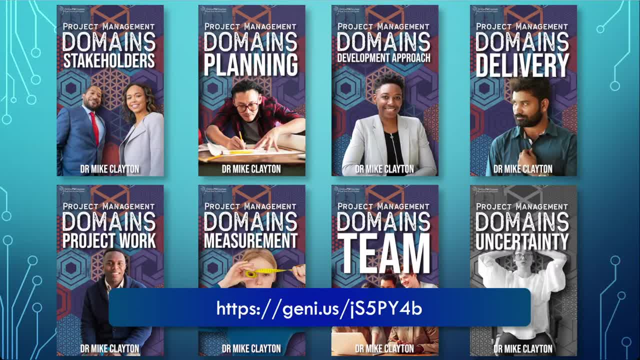 So we're talking about the how and the what rather than just the principles. The e-book set is available. In fact don't tell anyone, but I actually did publish because I've got a head over the summer. I actually did publish the uncertainty e-book. 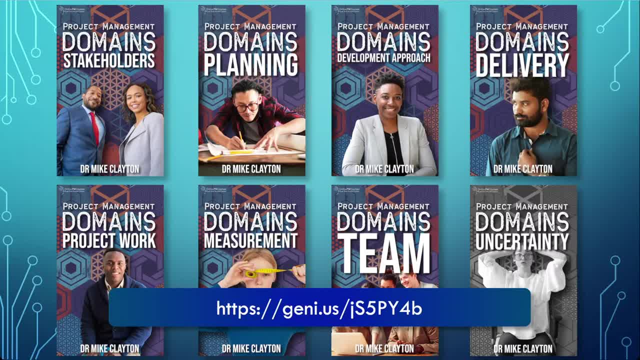 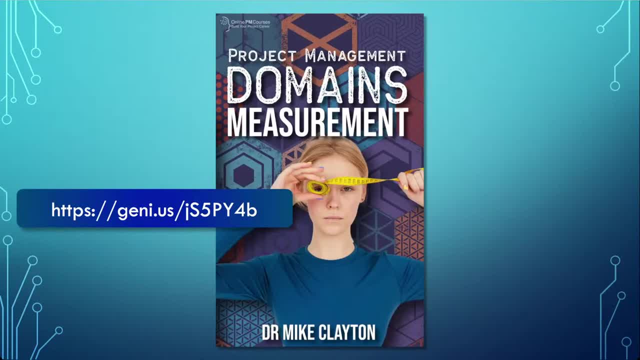 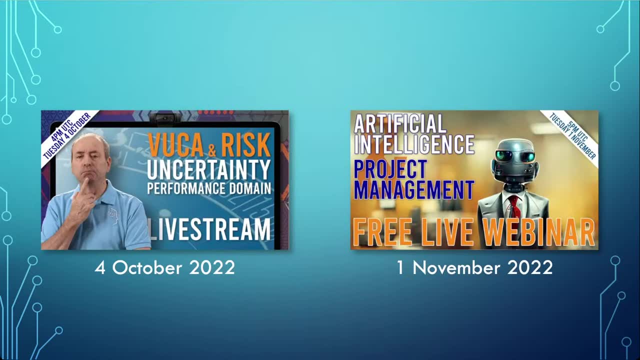 So the the set is available on Kindle. You can go and look at the set there. So that's the set. Say that, so go to the next slide. So this is the. this is the current e-book Measurement. I'm not going to kind of drag this out. 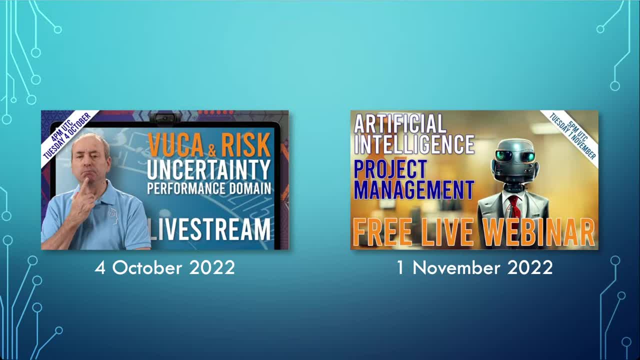 because it has been such a struggle for us all in my face, although it's really not that pretty. next week, fourth of next week, next month, fourth of October, first Tuesday in October, hopefully a stronger stream- We'll be looking at the uncertainty performance domain and the concepts of VUCA volatile. 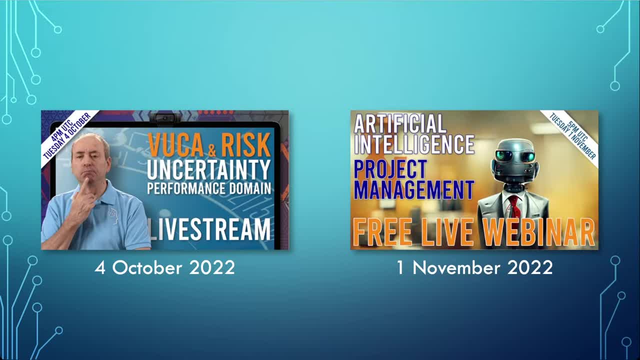 uncertain, complex and ambiguous environments That we work in and risk, And so that will be the last of our eight domain reviews, And so that I hope you'll enjoy that And then do something special. first November, I some of you will have attended a livestream- 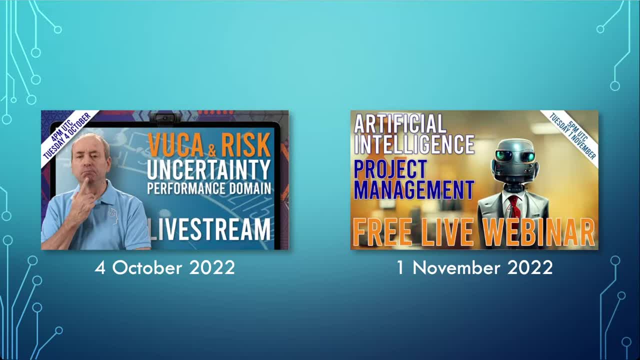 I did when I came back from the Association for project management conference. I think it was That that I said. I talked about the fact that I was planning to read about artificial intelligence and its place in project management Over the summer and I did and I got really interested in it and I thought there's a lot here that people want to know at the that livestream. 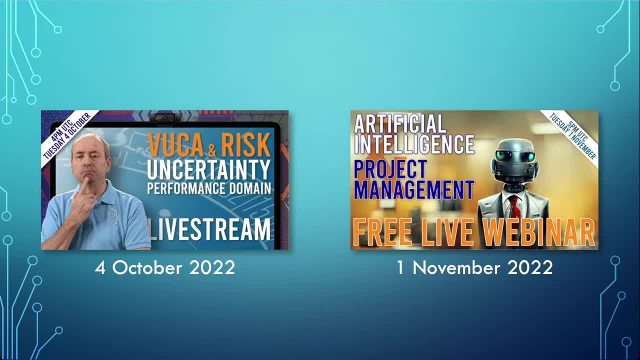 I think it was that livestream. I said who you know who would be interested in some content about the role of artificial intelligence in project management, and lots of people said they would. So first November- God, I hope we have a decent stream strength first November. 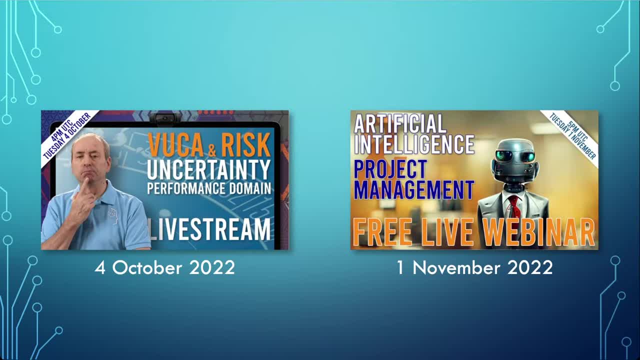 I will be doing a livestream, which is I'm good, but I'm going to be doing it as a free live webinar. I'm not going to be interacting with you as a group during the content delivery. I will take questions at the end. 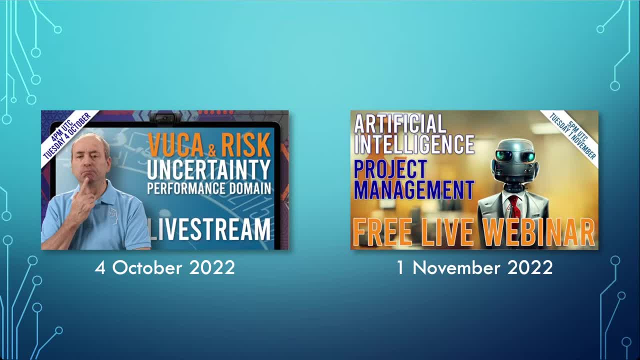 but we'll be doing on YouTube, So it will be free. I did contemplate actually having a paid webinar, But I think I want to do it free for you guys and that will be looking at everything I have learned about artificial intelligence: project management. 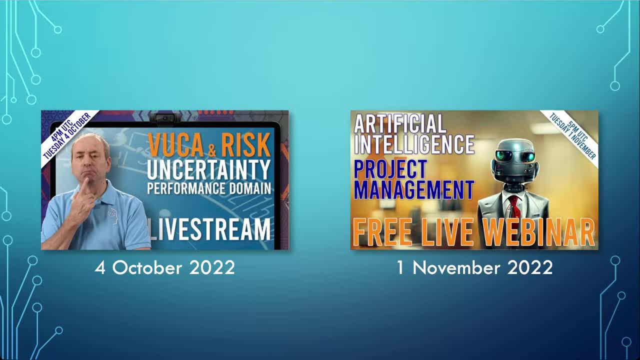 I'll be interested to hear your questions because those questions which, whilst I may not be able to answer them, may help me to frame an agenda for next year, for 2023, of learning more about artificial intelligence and perhaps getting some experts onto the channel. So save the date. 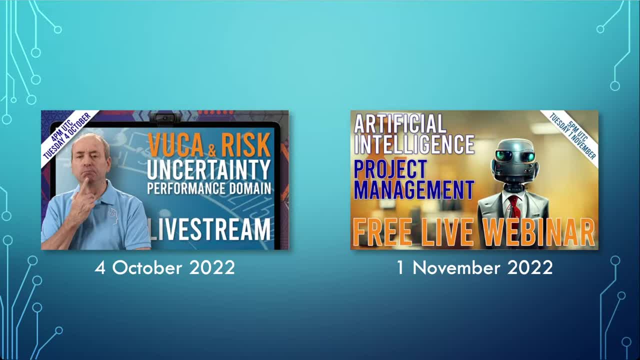 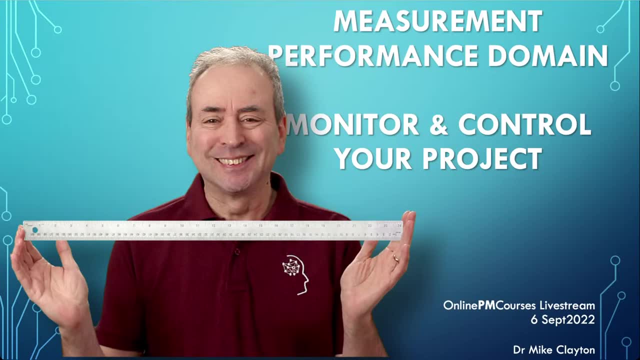 1st of November 2022.. We will be talking and it's for it's going to be. now It's 5 pm. My what these do ask any questions. I'm going to hang on. Hang on in said timing is is is tricky. 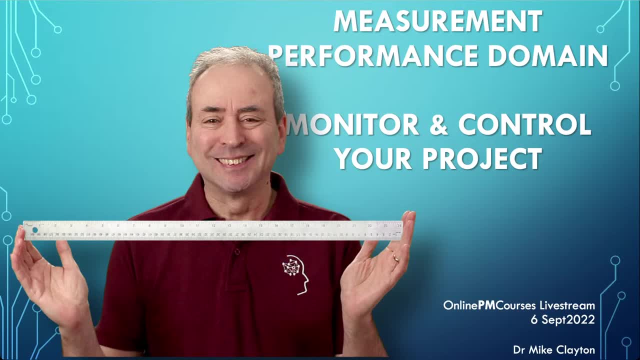 but I'm guessing it's something around the promotion for the future. Think Sunday wasn't talking specifically to you. It's just a coincidence of timing, I'm going to guess. But anyway, if you have questions, put them into the chat. 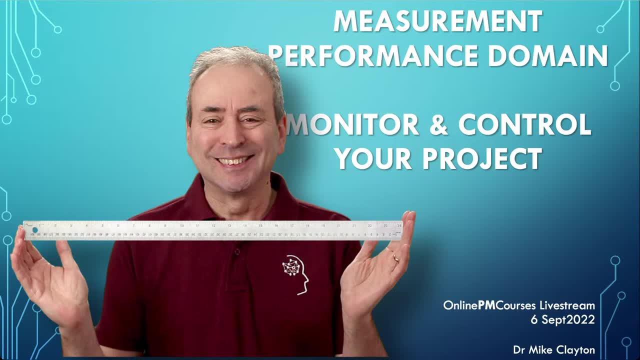 I'm not going to put my camera on because that will burn bandwidth and it's tough enough for the voice stream to get through. But those and then we will end the stream. Gerard, you're very welcome. Gerard says thanks for the presentation. 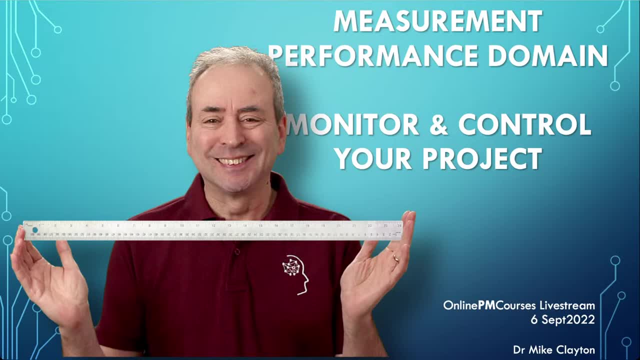 You're very welcome, Gerard, and stream and let you get back to your Lives, and I do once again apologize for the quality of the stream. It's been. it's been awful. I know, I know that I'm getting warnings all over my screen. 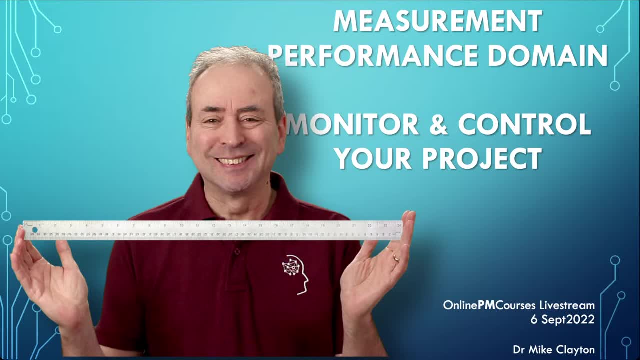 My bitrate seems to be averaging around about 1300- 1200. When it should be around four and a half thousand. So so YouTube tells me I will, and I've throttled it back. What I'm sending back to My mouse is behaving as well. 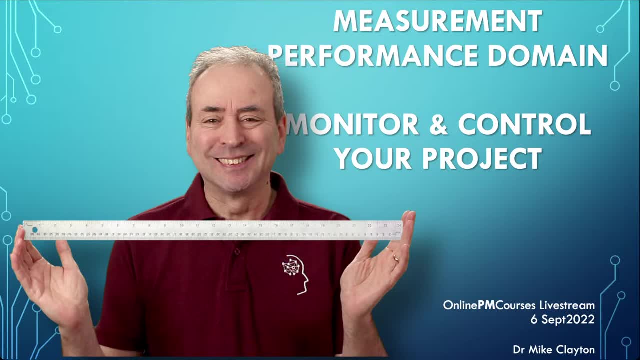 but that's just because my Where is my mouse? I can't see it Click something Here. we are throttled. So I've actually- Yeah, see, I'm sending it twice what it's actually going out at. So that's my, that's my internet. 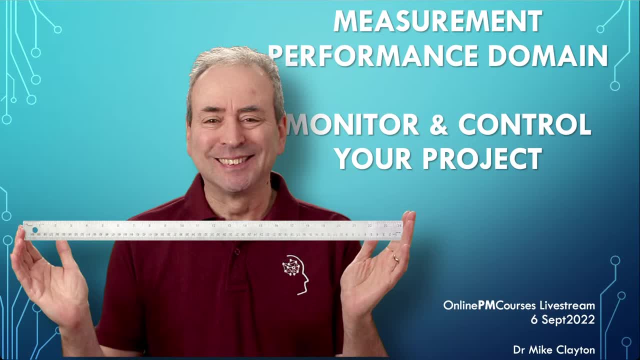 Okay, I've got nothing else in the chat, So I'm going to say goodbye. Sorry about the quality. Bye.